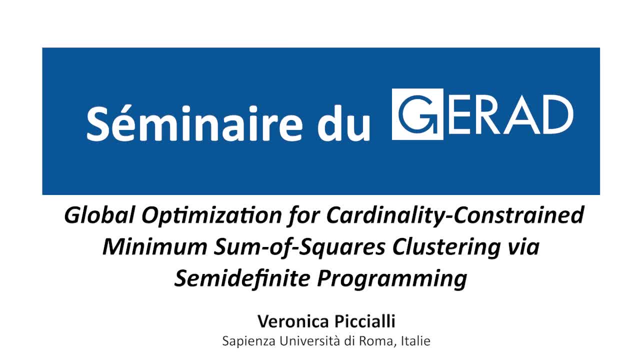 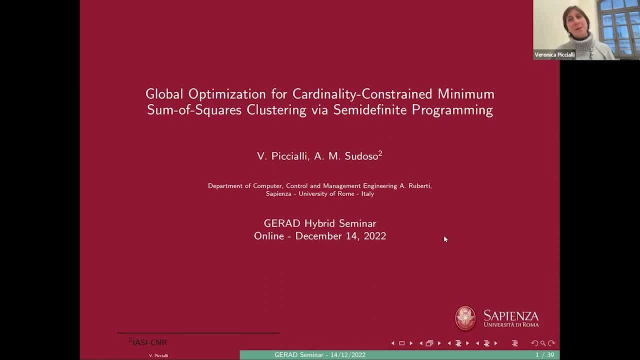 So this is basically this. what I'm going to talk today is mainly the last paper we wrote on clustering, which is the one on cardinality- constrained minimum sum of square clustering- But in order to give you an idea of why this problem is difficult and how we got there. So in the first part of the talk I'm going to talk about also about what we did for the unconstrained case and the pairwise constrained case. 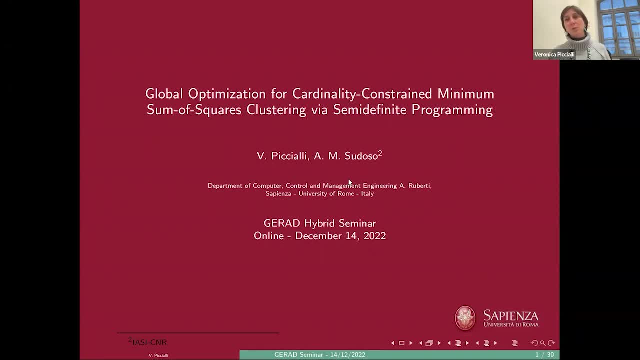 And so this is a joint work mainly with. Antonio Sudoso is the, my former PhD student, now is a postdoc in Rome at Iasi, And but there are some other people involved in the first part, which which are Angelica Vighele and Anna Russo-Russo and other PhD students. 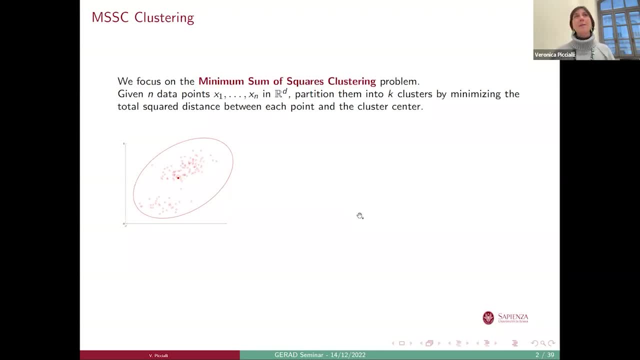 So the problem we are going to address today is the minimum sum of squares, clustering problem, And the idea is that we have n data points in our d, So we have d features and n points And we would like to cluster them. We would like to cluster them into k clusters and we assume that the number k of clusters is given. 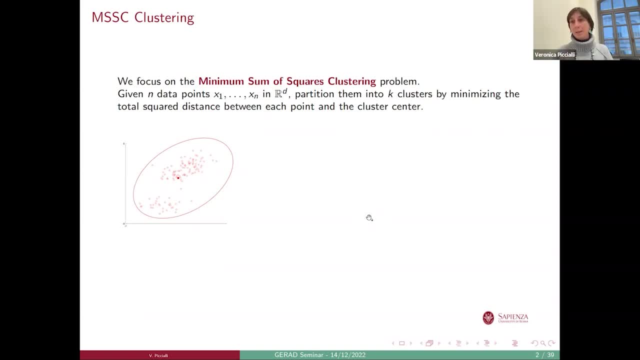 And the objective we want to minimize is the total square distances between each point and the sum of the total square distances between each point and the cluster center. So here you can see an example. if I have this set of points and I'm requiring to just one cluster- of course I'm putting all the points in the same clusters- is if k is equal to two. this is what I get. 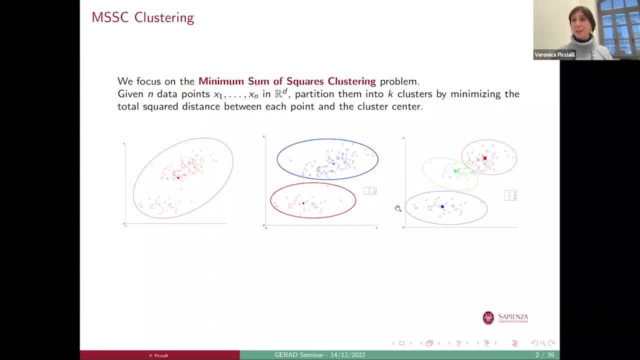 If k is equal to three. this is what I get. So here is the is the center of the cluster. So the objective we are minimizing is just the sum of the distances between each point and the cluster center. And it is known that if you have for a given cluster assignment, then the optimal cluster center is the average of the points in the cluster. 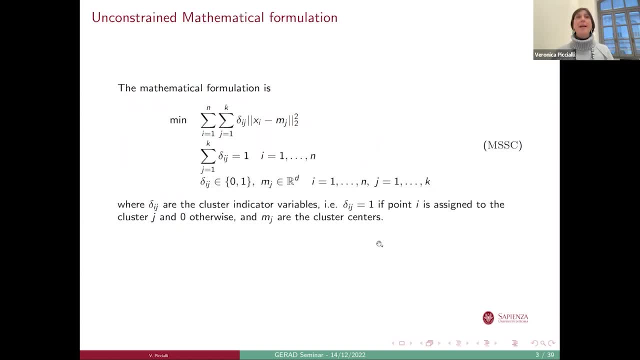 So it's basically the barycenter of the points in the cluster, And the straightforward mathematical formulation for this problem is this one, which is a mixed integer, nonlinear programming problem problem where we have as a variable the delta J, which are the cluster indicator variables. 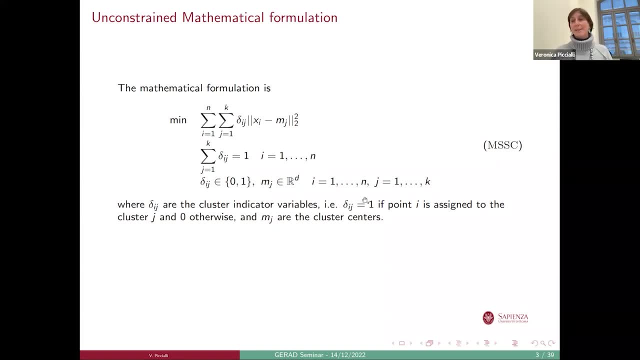 And that means that delta J is equal to one if point I is assigned to cluster J and zero otherwise, whereas MJ belong to RD, so have the same number of features of the point and are the cluster centers, And this problem is known to be NPR, even if we only have two. 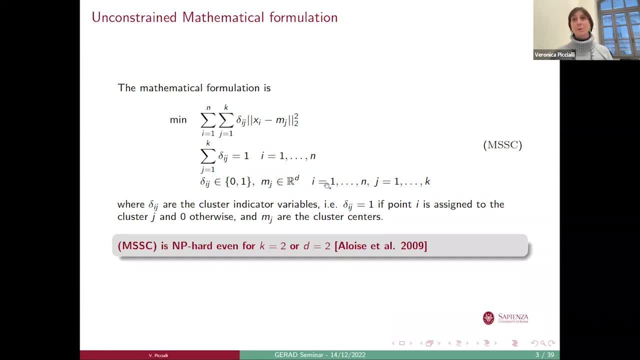 clusters, and even if the points are on the plane, So if D is equal to two. So this is a very difficult problem, And so that's why most of the literature for this problem tries to propose the heuristic algorithms. So, however, there is a reason for trying to look for the global minimum. 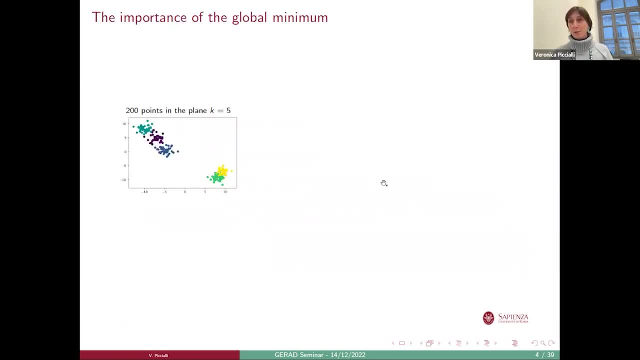 for this problem And in this picture I'm trying to give you a motivation. So we are in the field of unsupervised machine learning. That means that we don't have a ground truth. So we need to interpret the results and to understand whether we did a good job or not. looking at the 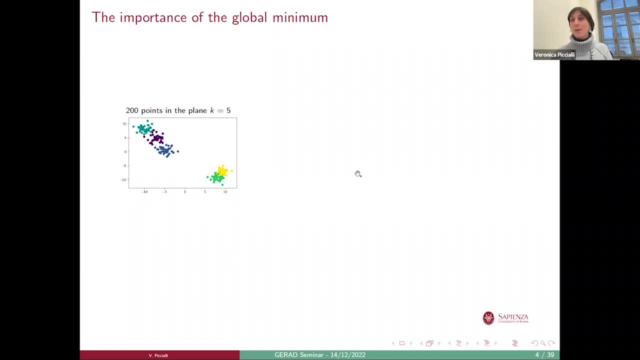 results. So we have to interpret the results without any error function that can tell us whether we are doing well or not. So if you take this, 200 points in the plane with k equal to five and you just run, k means a small like certain number of times, which is the most famous heuristic for this. 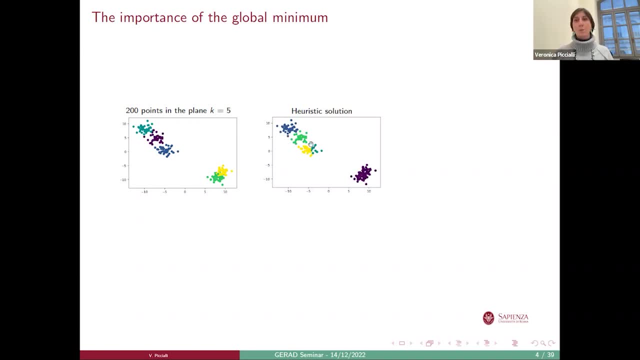 problem and which is the one I will discuss later. So you will see how I found this solution. This is the heuristic solution you get, And so if this is all you got, then you just should interpret the results Looking at this clustering you have here. But if I solve to the global minimum this problem, 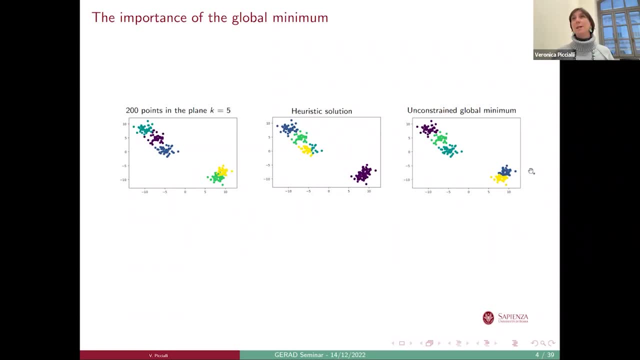 then I get a completely different clustering. So you see, the points are grouped in a completely different way. This implies that the interpretation derived by the heuristic solution might be completely wrong. So if I only have heuristic solution, I have no way to decide whether that 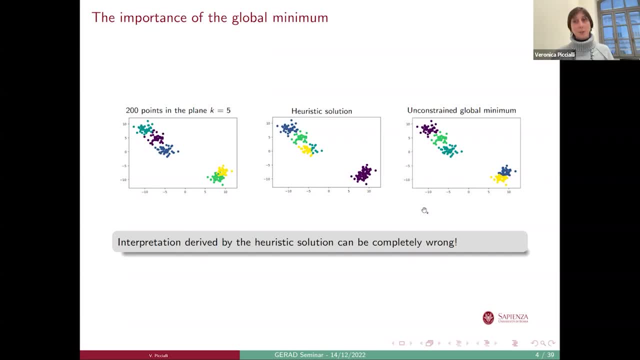 is a global minimum or not, And I don't know whether my interpretation is the correct one. So that's why I think it's worthwhile to investigate exact approaches for this hard problem, And so something else that one can do to improve the quality of the solution is to introduce: 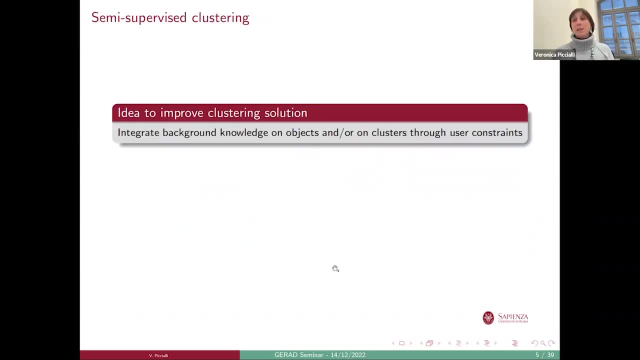 if available, some background knowledge on objects and or clusters, adding some constraints. And this kind of background knowledge can come, for example, from experts in the field that know for sure some information on the cluster, or from some requirement on the problem And, in particular, 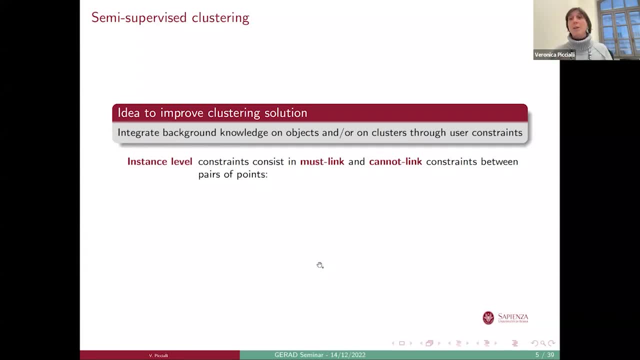 you can have instances Where you can have constraints. those can take some space time to get into in the action. So a clustering is very clear and stable And you can have some constraints on the addition of different point. pueblo of Mexico say in theEl Cluster Divide, for example in the 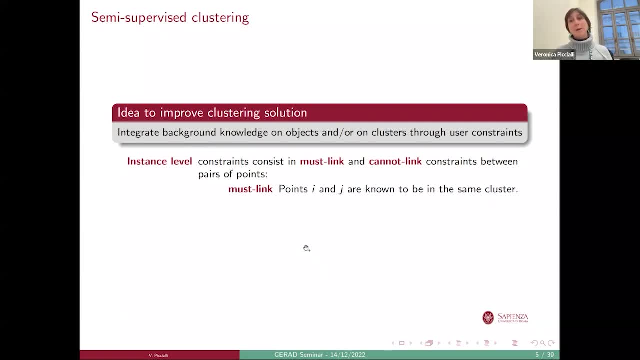 addition of different points sized so you can have at least dicencao and the separators in the thing, a multiple, classic way, you would cancel this clustering. And of course this is very important because we need some Python and CNN as the example. 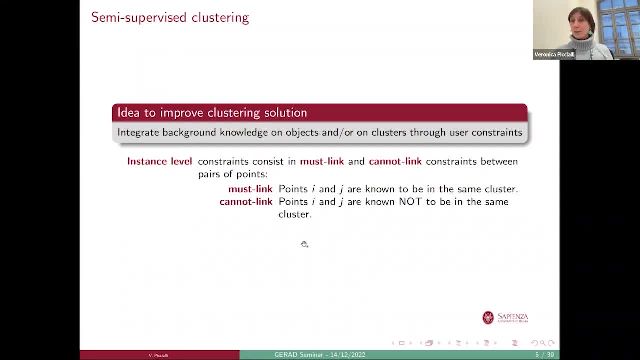 here Constraints, which means that you can have constraints that take a pair of points and decide whether they should be together or they should be separated in the final clustering. So you have a must link when two points- I and J- have to be in the same clusters, Or 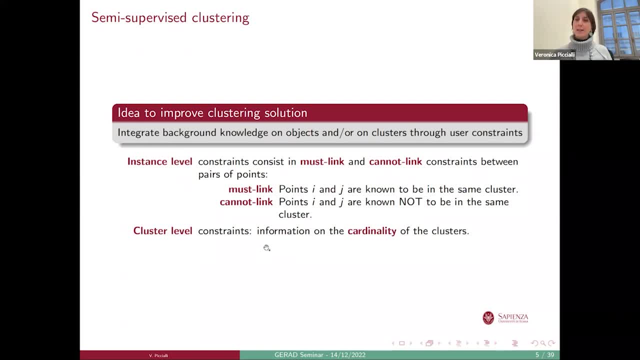 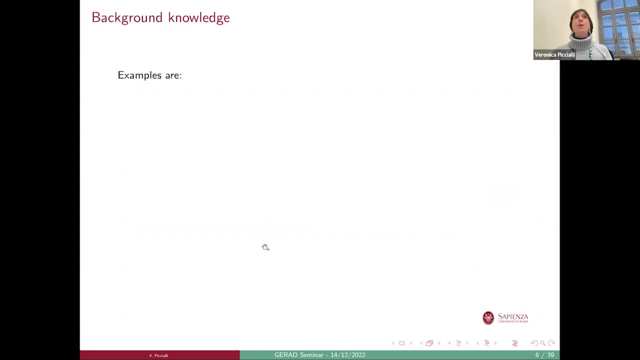 you have a cannot link when you're sure that point I and point J shouldn't be in the same cluster. information on the cardinality of the cluster. So, for example, you know in advance how many elements you will need to have in the cluster. So examples of constraints that one could add. 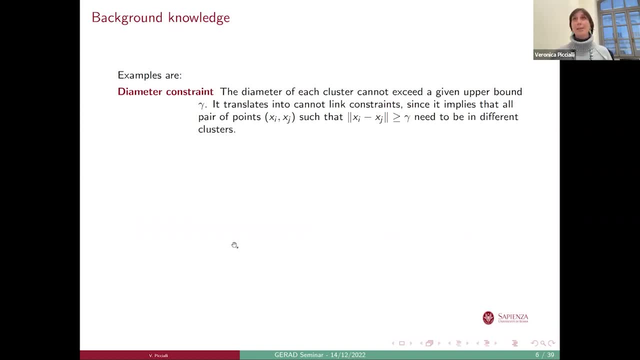 are diameter constraints. So in this case, basically, what you're saying is that you know by the structure of your problem that the diameter of each cluster cannot exceed a given upper bound. This means that if you have two points that are more far away than the threshold that you have, 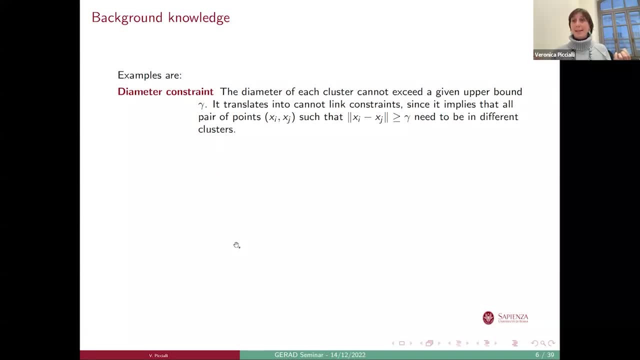 those two points cannot be in the same cluster. So this implies that I'm imposing some cannot-link constraints between points that are far away from each other. Otherwise one may have some split constraints, which imposes some lower bound on the separation between clusters. So 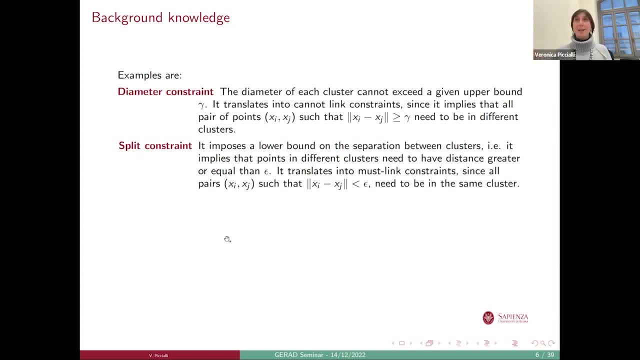 in this case, this implies that if two points are in different clusters, they need to have a separation between clusters. So in this case this implies that if two points are in different clusters, they need to have at least a certain distance. So this, on the other hand, 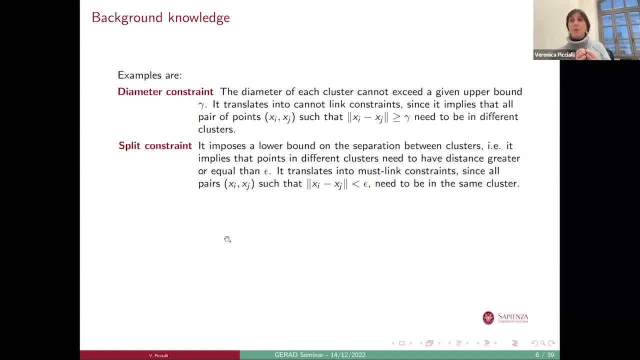 implies some must-link constraints, because if I have points that are really close together, I want them to be in the same cluster And so these two kind of constraints give me some pairwise constraints. So must-link and cannot-link If I have some cluster-level. 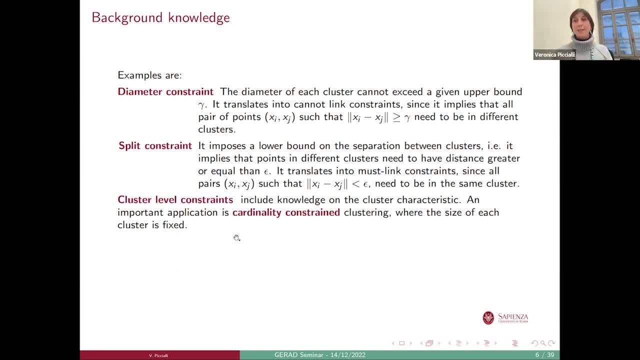 constraint. that implies that I have some knowledge on the overall characteristics of the cluster and an important application, which is the one I'm going to talk mainly today, is cardinality constraint clustering, where the size of each cluster is given. So what I know 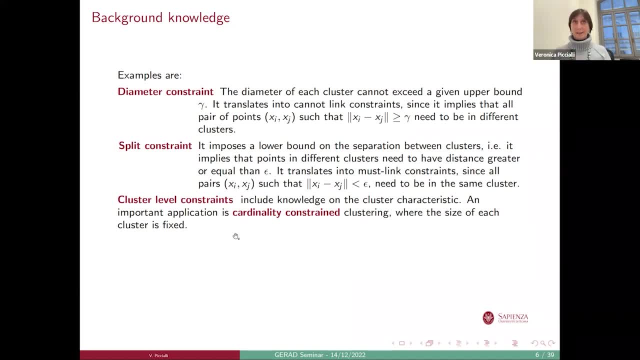 is for each cluster, how many points will be in that cluster? And the only thing that one should be careful about is that I have to be sure of the constraints I'm adding, because, of course, if I'm adding some inaccurate or conflicting constraints, then what I can do instead of 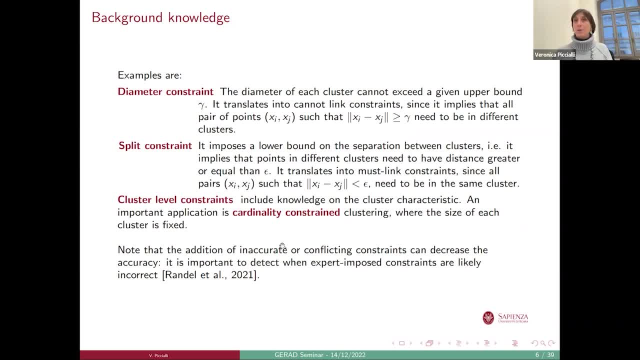 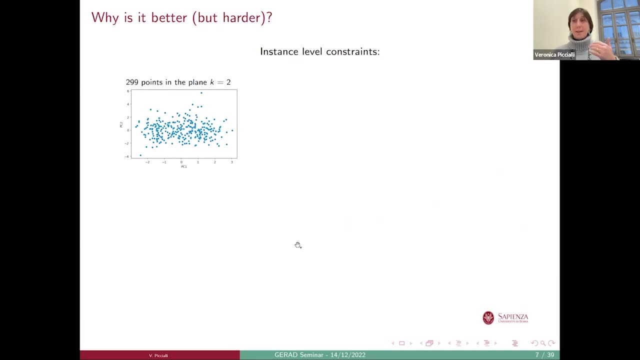 increasing the quality of the solution I'm getting is getting a worse solution. So it is important to detect whether some expert-imposed constraints are in the same cluster, And so this is a good idea, because if I have this information, I can improve the quality of. 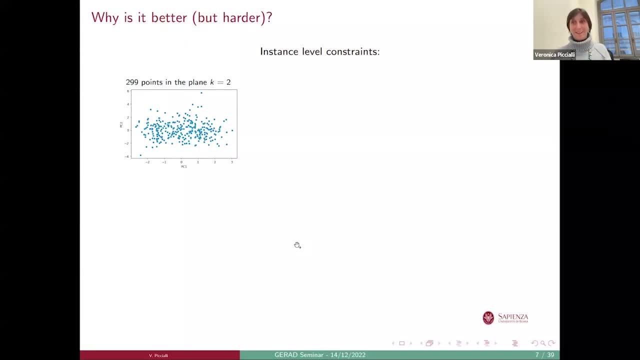 the solution, But on the other hand, it makes the problem even harder. So I'm just going to give you another example with another picture. In this case I'm talking about instance-level constraints. So I'm assuming that I have must-link and cannot-link constraints And assume 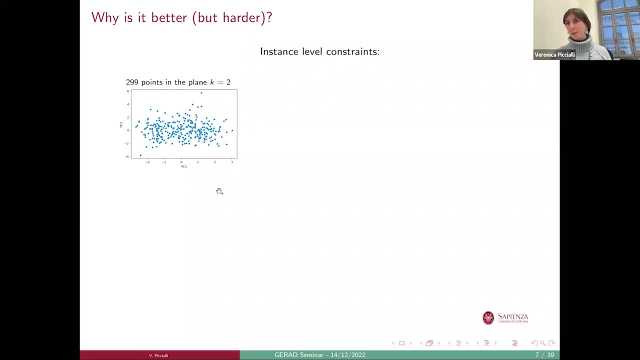 that this is my dataset. So these are the points again on the plane so that I can draw them, And this is the real ground truth, which I don't know. I have two clusters and this is the ground truth I would like to reach If I solve the unconstrained global minimum. this picture is: 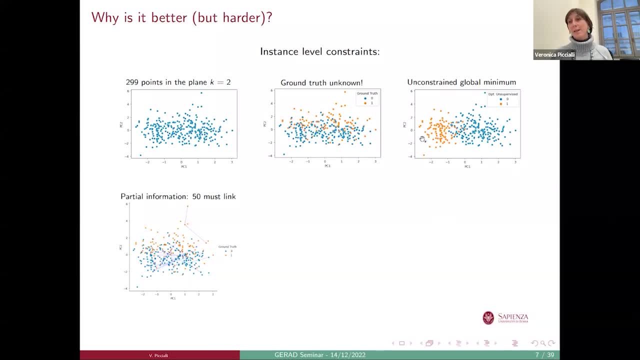 what I get And, as you can see, the objective function of k-means drives me sorry of the minimum sum of squares. clustering drives me towards two clusters that are kind of spherical and that are kind of separated as possible. But then if I add some information like, for example, 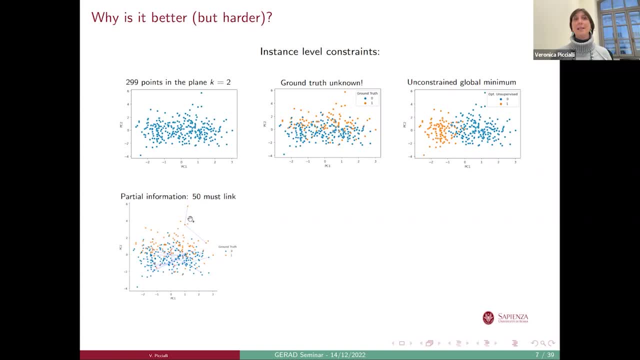 I have some constraints, some must-link constraints- let's say that I have 50 must-link constraints- and then I have some cannot-link constraints, like these ones I have in the picture, and then I solve the constrained version to global optimality. then, basically, I almost rig over the ground. truth: 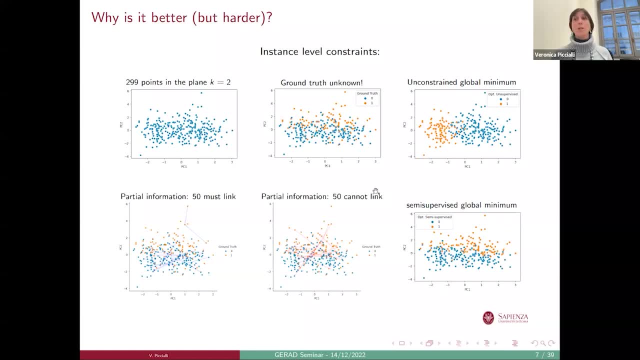 So adding the information gives me a much better quality of the clustering, But on the other end, if you think about it for a second, my objective function would drive me to this solution, whereas I'm looking for this one, So it's harder to find. 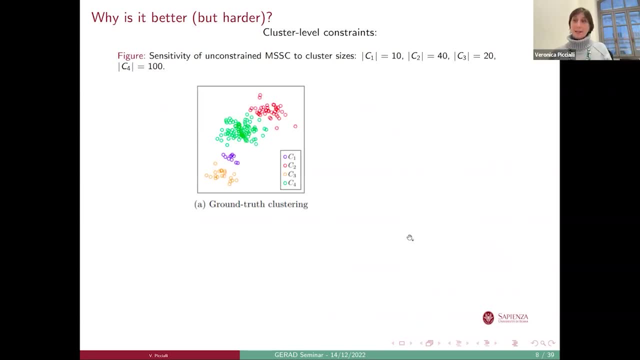 That was pairwise constraint. If I go to cluster level constraint, like, for example, the cardinality, again assume that this is the ground truth: clustering okay. But if- well, you see that I have clusters of different cardinalities, Well, if I solve the unconstrained version of the minimum, 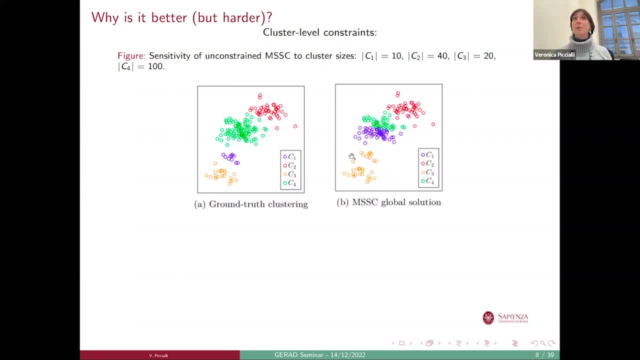 sum of squares clustering. what I get is this global solution that, as you can see, is kind of far away from the ground truth. So if I solve the unconstrained version of the minimum sum of squares, what I get is this global solution that, as you can see, is kind of far away from the ground. 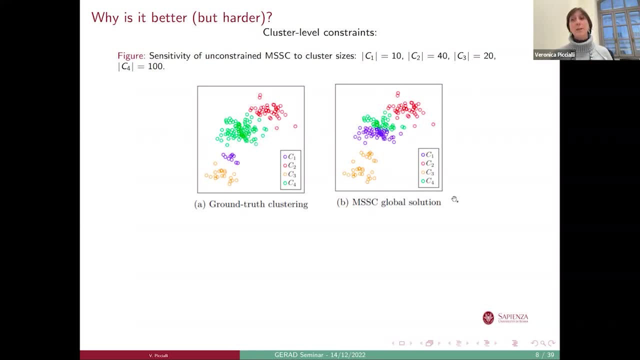 truth. But if I add the information that I know, what are the cardinalities of the optimal clustering? and again, I'm going to solve to global optimality my problem. so I'm always assuming now that I'm solving the problem to global optimality, because that's what I'm. 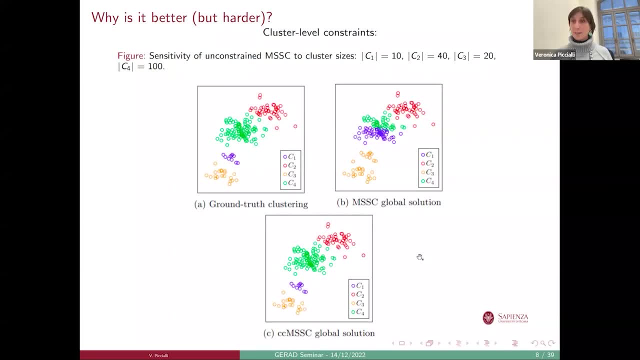 interested in doing. then you can see that I basically recovered the ground truth. So adding background knowledge improves a lot the quality of the clustering, but that makes the problem harder. So I have to think, and we will see that, whether on the one end I could 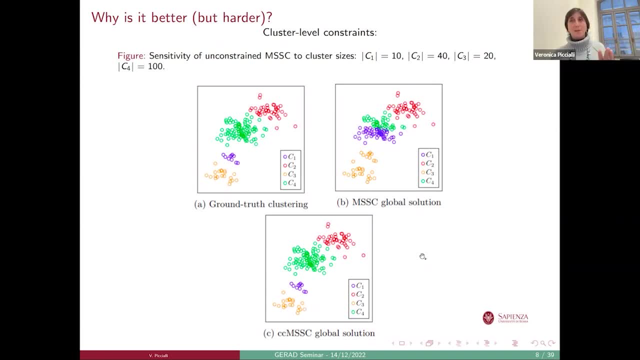 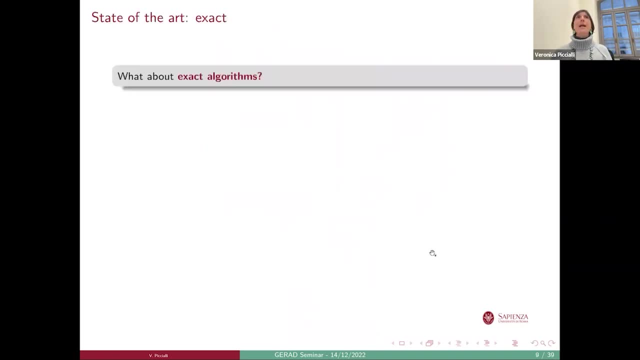 somehow do the same thing for the unconstrained and pairwise constraints. When I introduce cardinality constraints, I need to do something significantly different. So what is the state of the art in the literature for exact algorithm for clustering? Well, if I go to unconstrained, it is known that it is a mixed integer nonlinear programming problem. 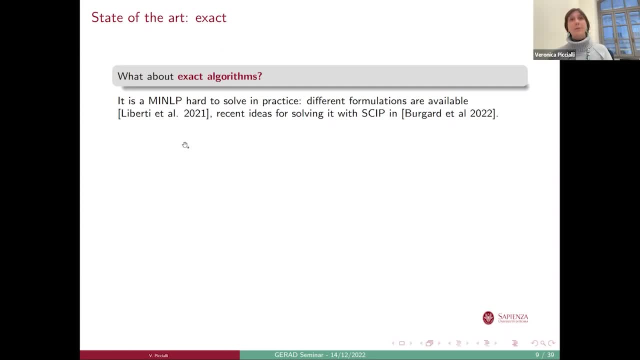 that is hard to solve in practice. I have some different formulation and there are some recent ideas for solving the original formulation which we ship in this paper. but in general it is extremely hard For the unconstrained version of the minimum sum of squares clustering right now. the state of the 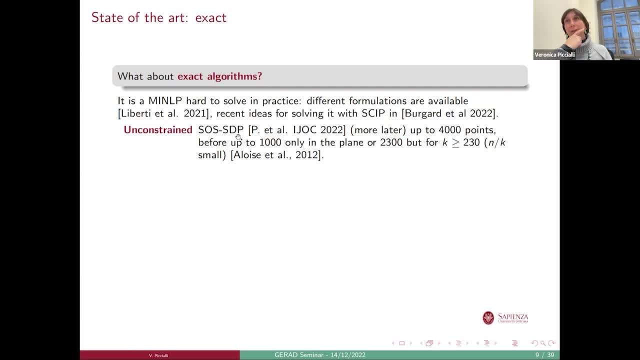 art is our algorithm, which is based on semi-definite programming, and it is the first algorithm that is able to solve, to global optimality, instances up to 4000 points. Before one could solve up to 1000 points in the plane and 2000 points, but only for a large number of clusters, which 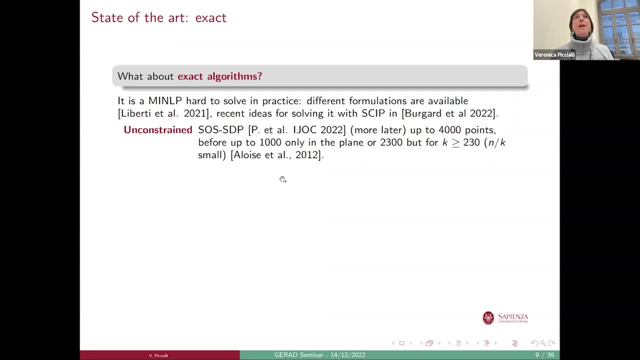 usually in practice is not that interesting For distance-level constraints. we were able to extend the algorithm we have defined for the unconstrained case and for the first time we were able to solve instances up to 800 data points, whereas before the state of the art. 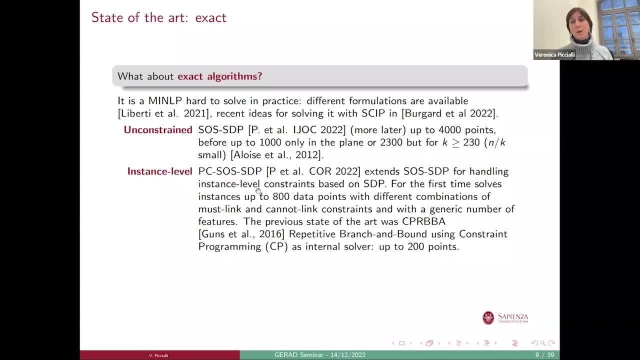 which was a repetitive branch and bound, could only reach 200 points. Again, this is based on SDP, so I'm going to give you some hints on how these two algorithms work For cardinality-constrained problems. in principle, any constraint programming-based 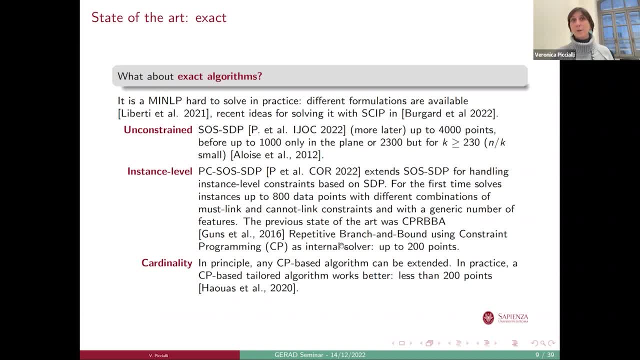 algorithm could be extended in order to handle also cardinality constraints, but in practice the state of the art is a tailored constraint programming algorithm but again it is able to solve to global optimality only instances with less than 200 points. All the other literature is basically heuristic and mainly on the unconstrained and instance-level. 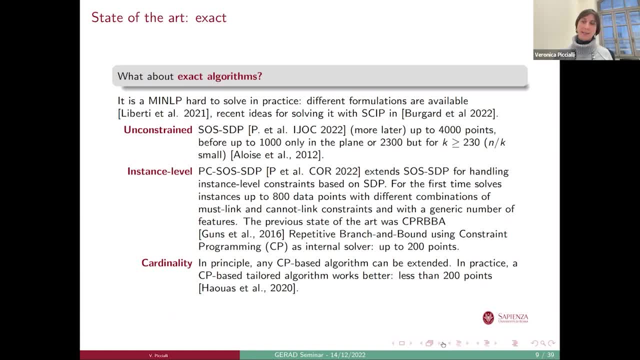 constraints. On cardinality, there is not that much, even on the heuristic case. the only case that is a bit more, let's say, considered in the literature is the case where we will see which is a special case, which is the balanced case In the balanced case. 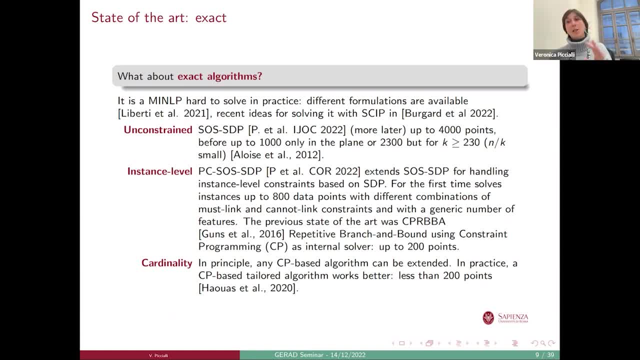 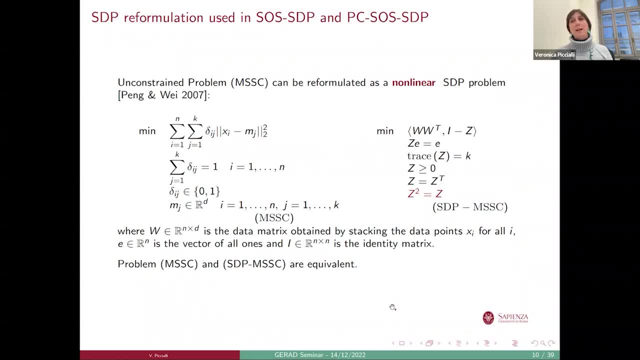 all the clusters have the same cardinality and so for that special case there is some literature dedicated. So the two first methods- I told you the state of the art- that are based on semi-definitive programming, both rely on a reformulation. 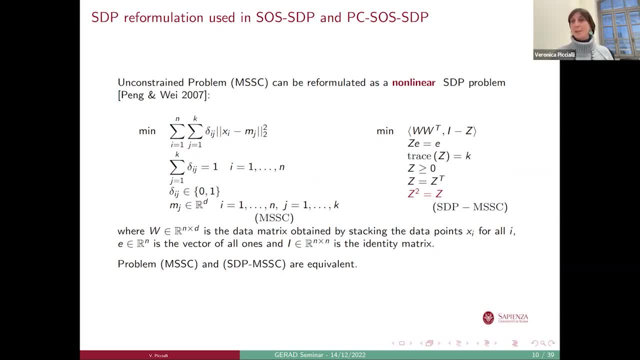 of the unconstrained minimum sum of squares, clustering based on semi-definitive programming. And what has been done? is was done in 2007 by Peng and Wei. what they did is to reformulate the mixed integer nonlinear programming problem as a nonlinear SDP And, as you can see, 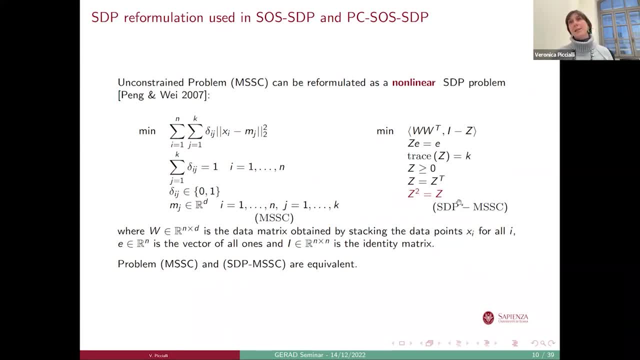 the source of nonconvexity here is the nonlinear constraints, z squared equal to z, And this matrix W is just the matrix obtained by stacking all the data points in, on on on of the data set. And these two problems. 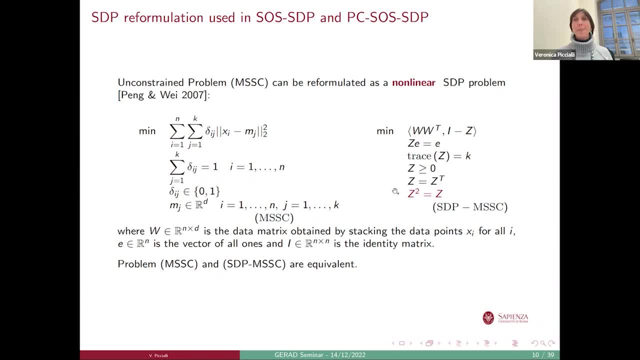 are completely equivalent. So this is a reformulation, okay, And this is also called the zero-one SDP, the Peng-Wei zero-one SDP. Starting from this SDP, a relaxation has been derived. that is called the Peng-Wei relaxation, And what is interesting is that for this problem, 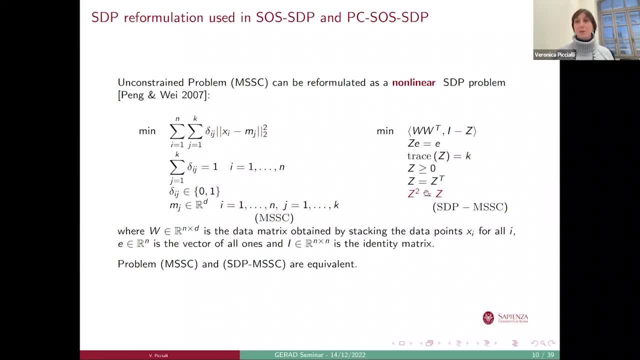 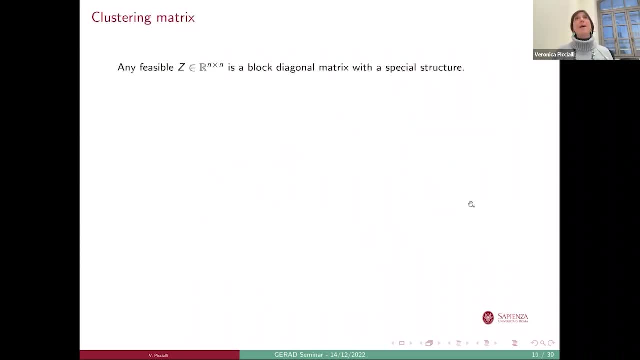 the matrix variable z has a very special structure. So my matrix variable z here has a very special structure. That is, it is a block diagonal matrix And whenever I have- Sorry, I don't know, Okay, Whenever I have- two points that are in the same cluster C, what happens is that the matrix 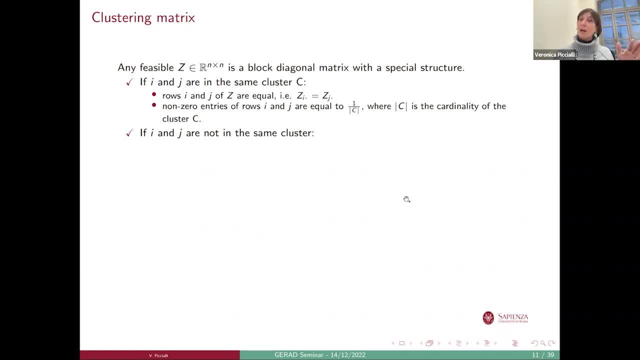 z has two rows that are equal. so the rows row i and row j of matrix z are the same. Not only, The non-zero entries on those rows are all equal to one over the cardinality of that cluster. okay, And if i and j point to z? 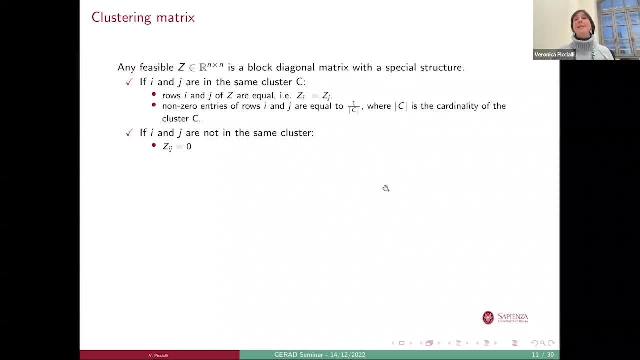 points i and point j are not in the same cluster, then the entries that j will be equal to zero. So this implies that, if you think about it for a second, that I can impose pairwise constraints on this formulation quite easily, because you see that I can impose- the two rows are equal if I want. 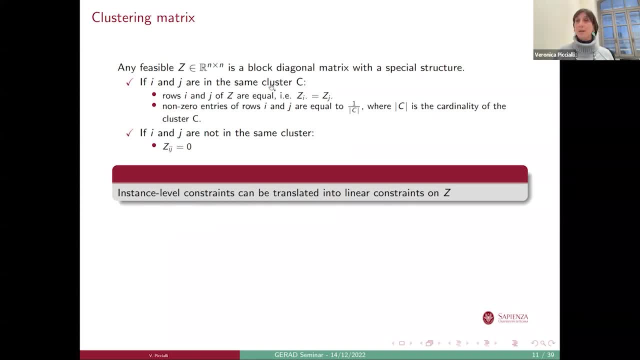 to impose a mass-linked constraint- and this is just a linear constraint, or I can impose that the elements that j is equal to zero if I have a cannot-linked constraint. So in this formulation it's kind of straightforward to impose instance-level constraints, since they just 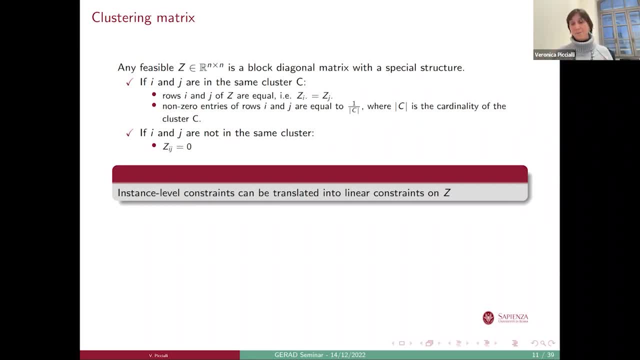 translate into linear constraints on the elements of the matrix Z. To give you a better idea, if we have six points that are divided into three clusters, so I have x1 alone. so cluster 1 is cardinality 1.. Cluster 2 includes points 2 and 3, and that's cardinality 2.. x4,, x5, and x6 are 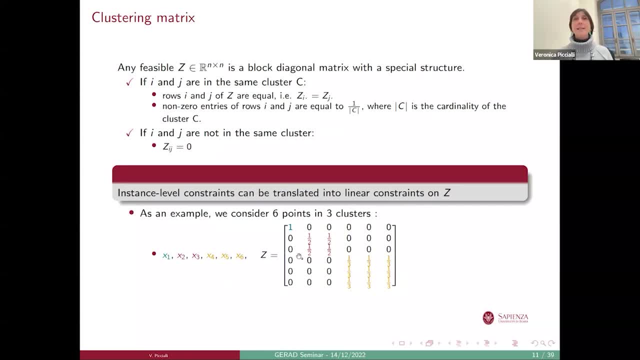 together in the third cluster, so we have cardinality 3.. This is how the matrix will look like. So if we have x4, x5, and x6 together in the third cluster, so we have cardinality 3,. this is how the matrix will look like. So if we have x4,, x5, and x6 are together in the third cluster. 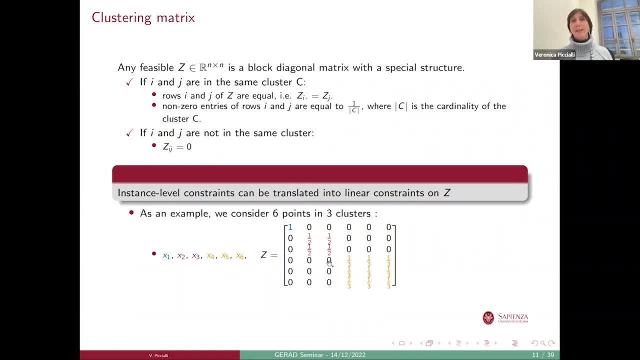 so we have cardinality 3.. This is how the matrix will look like. So you see, it's a block diagonal matrix and you have the elements. the rows are the same for points that are in the same cluster, whereas when two points are not in the same cluster, the element is zero. But you can see. 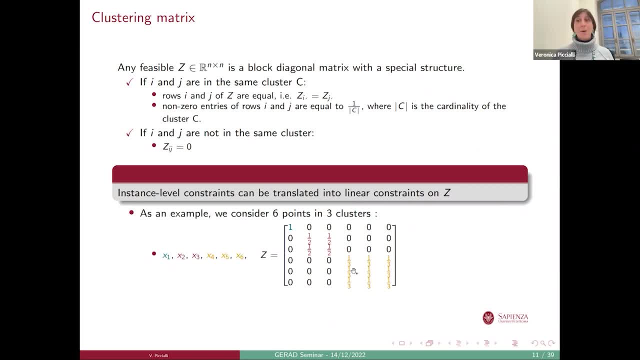 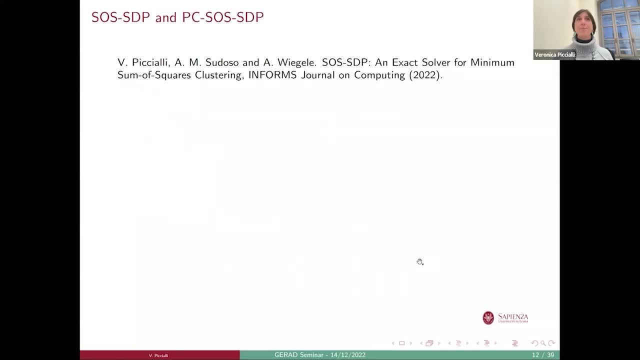 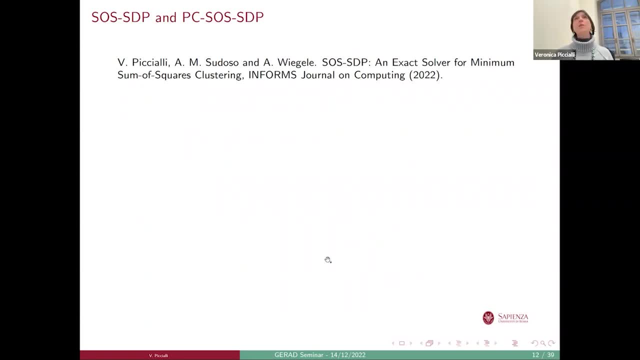 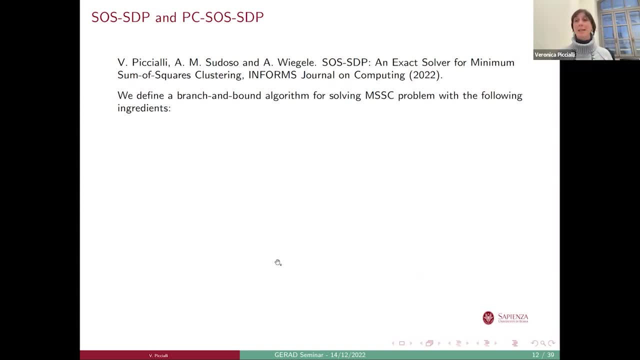 minimum sum of squares, clustering and the ingredients we used. base was an SCP relaxation that is derived from the reformulation I showed you just now, But we strengthened and that was really fundamental And we will see that we're going to use that idea here as well. We strengthen and we, on the other hand, 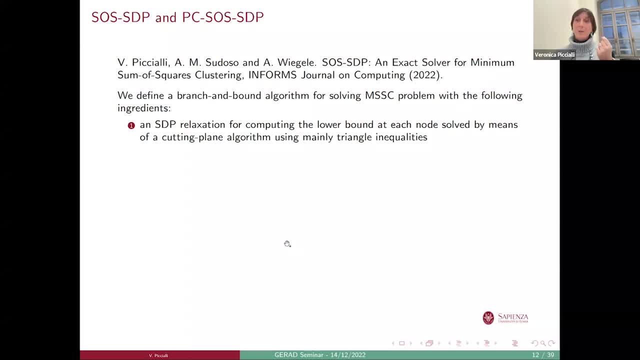 maintain the bound by a cut-in-plane algorithm. So we were adding triangle inequalities to make the bound stronger, And that was really one of the key elements. So having a strong bound was what allowed us to have a very good algorithm, And then we had also a primal heuristic to compute an upper bound. 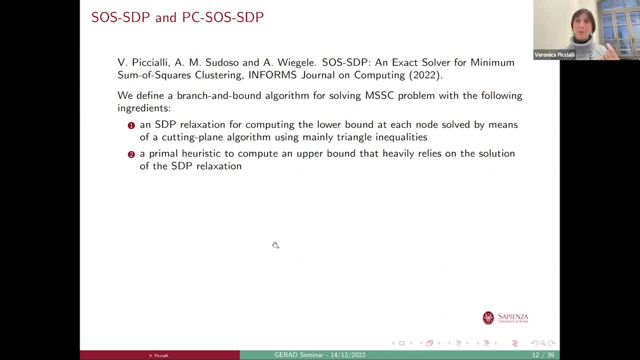 And again this primal heuristic heavily relies on the solution of the SDP. So again the good quality of the solution of the lower bound problem would allow us to get also a very good heuristic that can be used also on its own with some optimality guarantee. And then also we use a branching rule that is strictly related to the problem. 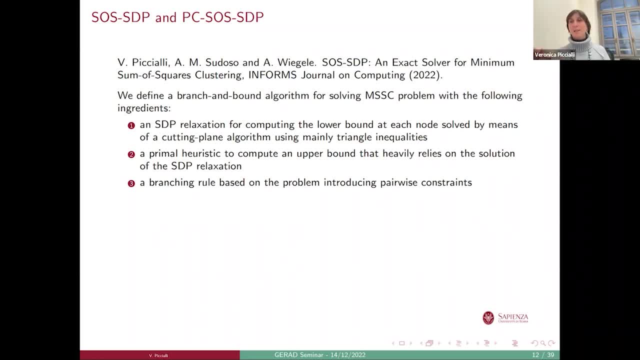 And we will see. it's the same we used here. So I'm going to get into details of that. And basically the way we partition the space is we take a pair of points and then we say, OK, either this or that These two points will be together in the final clustering, or these two points will not be together in the final clustering. 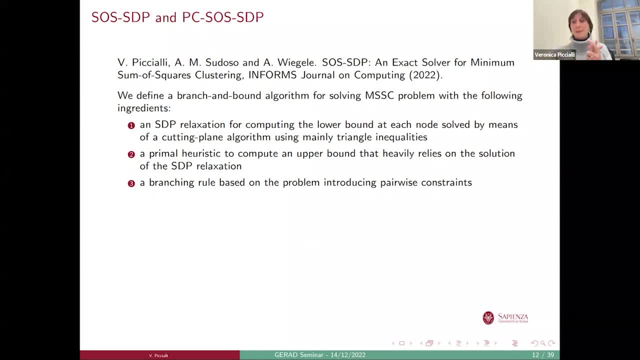 So you see that branching, the branching rule, imposes some pairwise constraints. On one child I'm saying those two points will be together, so I have the mastering constraints, And on the other child I will have. these two points cannot be together. 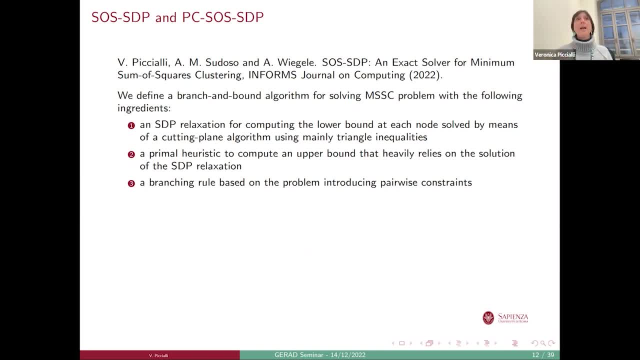 And in this case I'm going to have a cannot-link constraint. We extended this algorithm in a paper. This is a paper- This is the one you see here- that was accepted on computers and operations research, And here, basically, what we do is we extend the approach to handle pairwise constraints. 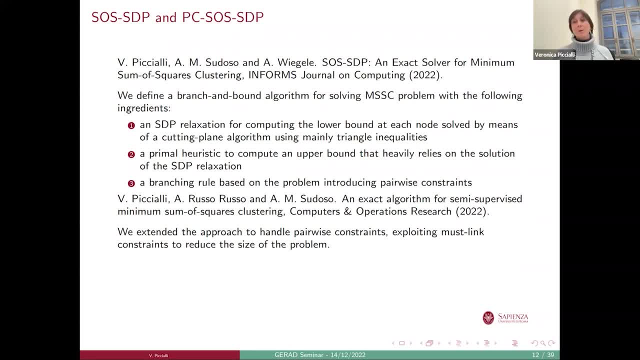 And mainly, we managed to exploit the mastering constraints to significantly reduce the size of the problem, And so this helped us a lot in finding and defining a good branching bound algorithm. also, in this case, And again, the ingredients were the same, So we were using a strong SDP relaxation. 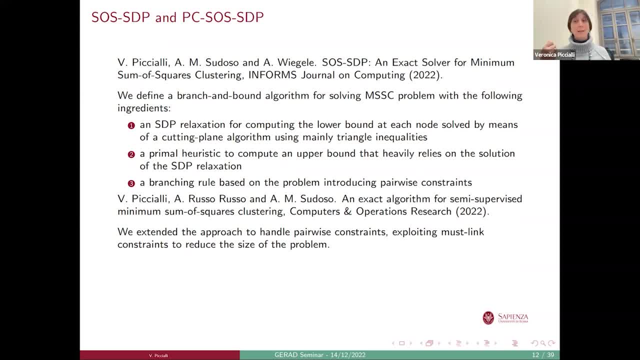 We extended the heuristic in such a way to handle also pairwise constraints And we were able to really take advantage of the mastering constraints in such a way to reduce the size of the SDP problems we were solving. So one could say, OK, well then what you did is just extend what you did for the other two cases for cardinality. 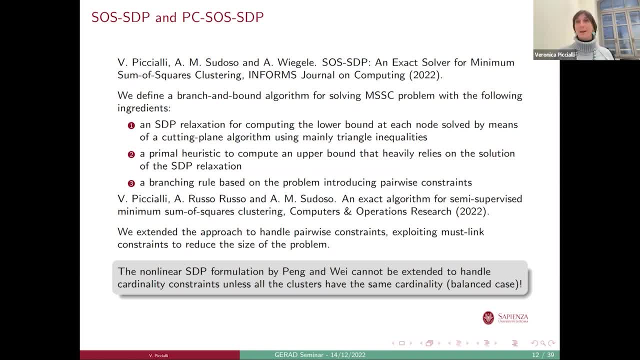 Well, the truth is no, because we could not use the Pang and Wei reformulation Because in that case, as I told you, the cardinalities are hidden in the problem. So I cannot impose explicitly constraints or the cardinality. It's something that I cannot do. 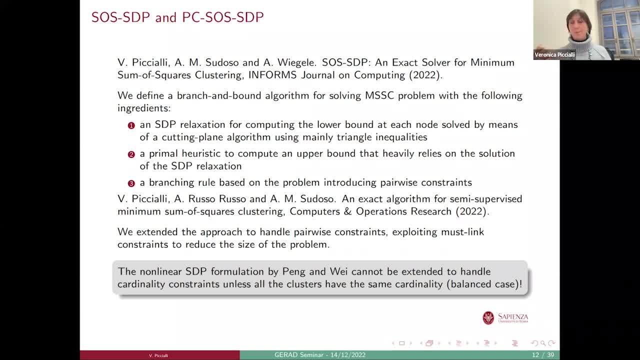 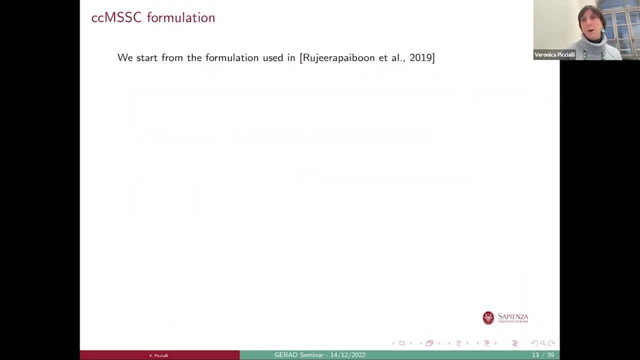 So I need to use a completely different formulation of the problem, And so what we did is we started by a formulation that is used in this paper, which is published on Cocteau in 2019, where they define a formulation for the cardinality constraint problem. 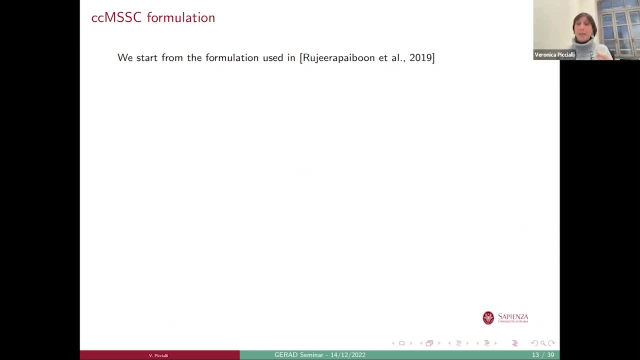 And they use this formulation Actually for for defining a heuristic and for doing bounding on the cardinality constraint, the minimum sum of squared clustering problem, And so what the I'm going to describe you, the formulation you have. C1, CK is just the number of elements in cluster one, cluster two, cluster K. 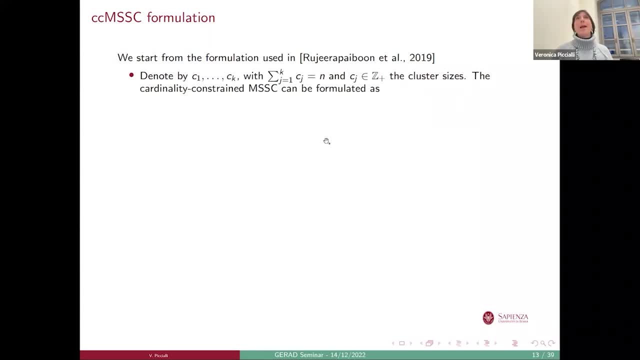 And so they represent the cluster sides. And then this is my formulation, where my decision variables now are these vectors: P by J. What is by J? Basically, for each cluster I have a vector that has the same length of the number of points, and that is just the cluster indicator. 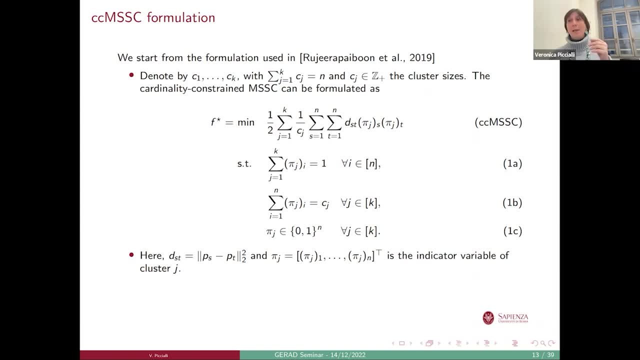 So I will have that by J. I will be equal to one if point I is in cluster J And, as you can see, these are binary variables And in the objective function you will have this term, DST of by J, which basically tells you the distance. 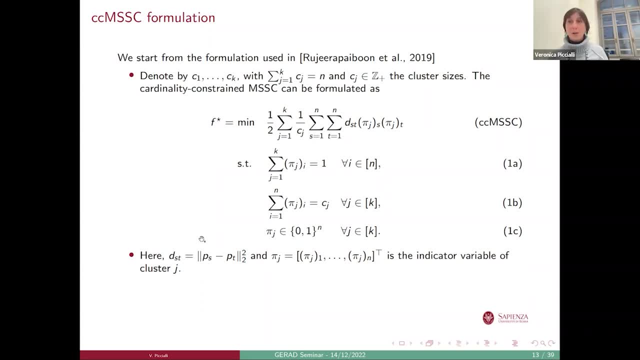 The Sorry that DST represents the Euclidean distances between point S and point T. So you can see that you have the difficulties hidden in these binary variables, of course, And it is known that even for the cardinality constraint case this problem is NP-hard. 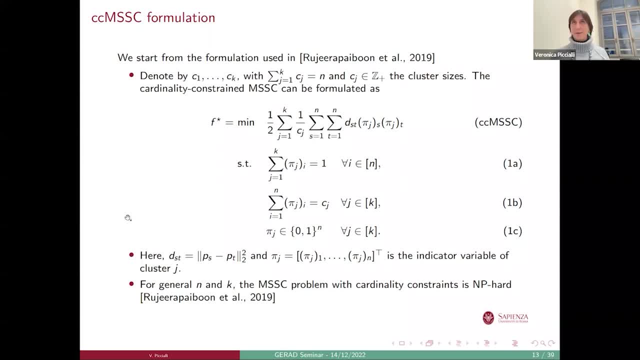 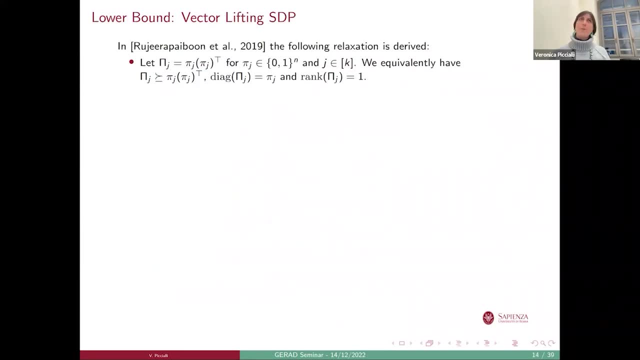 So the authors prove that the NP-hardness stays the same even for the cardinality constraint version. So what the authors do, So one thing: What they do there, they derive an SDP relaxation and an LP-NSTP relaxation, And they do this by doing some kind of matrix lifting. 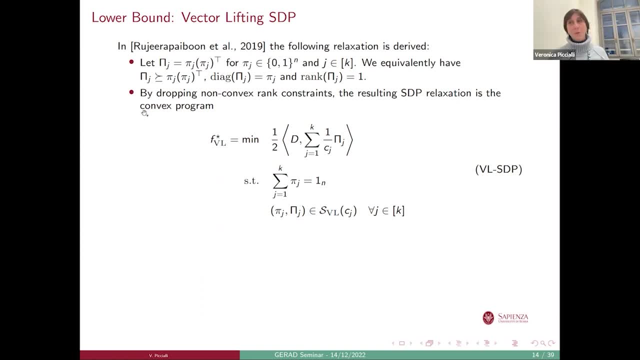 Because what they do is they define a capital- pi pi J- which is like a matrix that should be equal. The optimal solution should be equal to pi J times pi J transpose. But what they do is they relax the equality constraints with using introducing a positive semi-definiteness constraint. 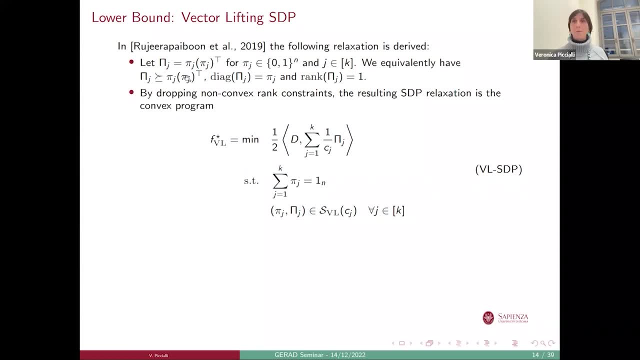 And this can be translated Basically by the Schur complement in the positive semi-definiteness of a larger matrix of size n plus one. And, as you can see, what happens here is that each of these metrics as size n times n. And then I'm going to. 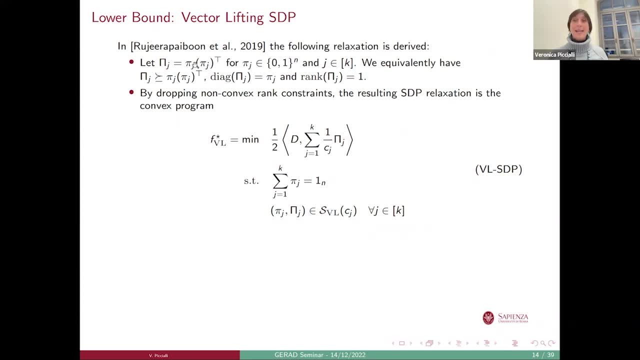 So what happens here is that I'm having as variables k matrices of size n plus one where k is the number of clusters, And when you drop- So you have equality, You are reformulating the problem If you impose that the rank of the matrix is going to be one. 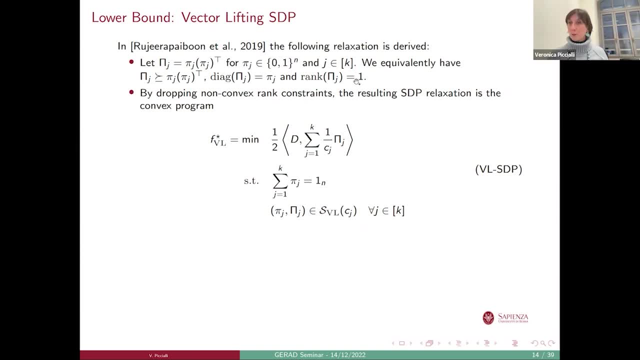 If you drop the rank one constraints, then you get of course a relaxation of the problem, And this is an SDP. This relaxation has been introduced in that paper And this set is defined in this way, where you can see that here I'm imposing the cardinality constraint. 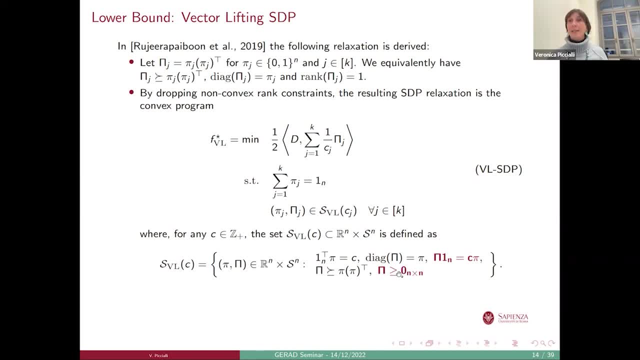 And I'm also strengthening the relaxation by adding that the elements of the matrix pi need to be non-negative. So this is a doubly non-negative relaxation, Because I'm intersecting The positive, semi-definite cone with the non-negative cone And we call this relaxation. 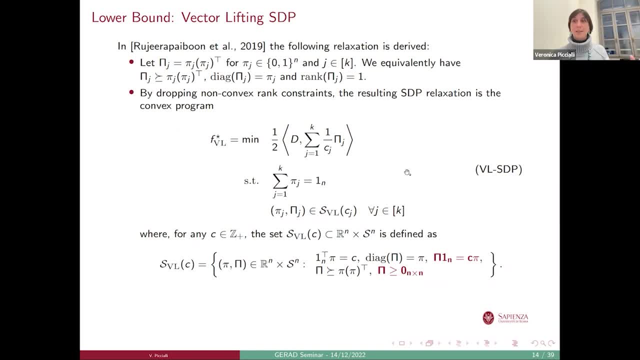 So the relaxation has been defined in that paper on SeaOpt in 2019.. And here I'm going to call this relaxation the vector lifting SDP. Okay, And as I was telling you, this SDP relaxation has k matrix variables of size, n plus one times n plus one. 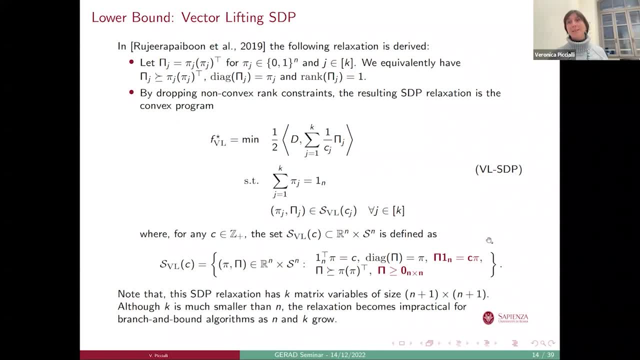 So even k is much smaller than n, then this relaxation becomes impractical When n and k are the same, When n and k grow at the same time. Okay, So this is why we tried, since we were thinking about defining again a branch and bound for this problem- 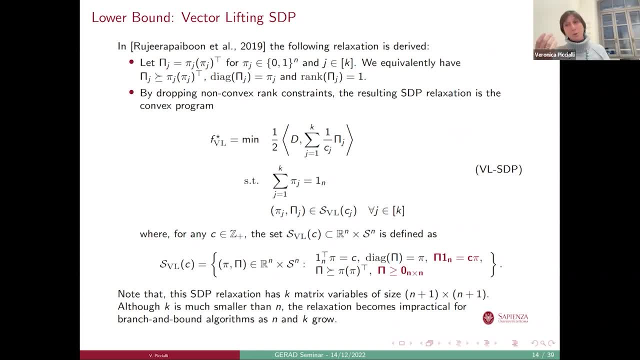 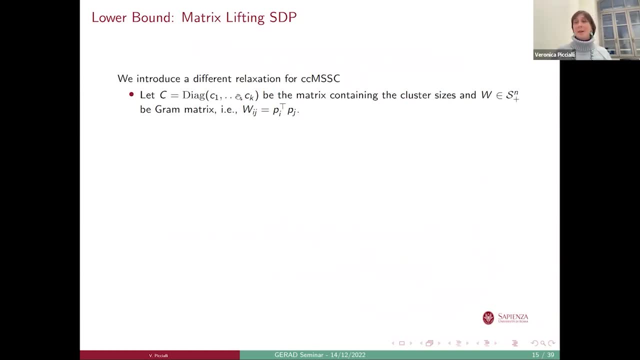 We were thinking about defining a different relaxation with which could scale a bit better, And that's what we did. So we, if we define, by C, the diagonal matrix, having on the diagonal the cardinalities of each cluster, And by this matrix, W, the gram matrix of the points, 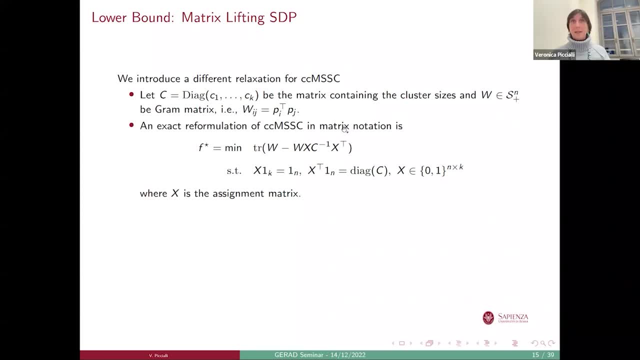 We can reformulate exactly the cardinality constrained minimum sum of squares, clustering in this way. And so what do we have here? The matrix X is a zero one matrix that represent the assignment matrix, So that will have n rows and k columns And we will have that. the element on the row high, the element j, will be equal to one. 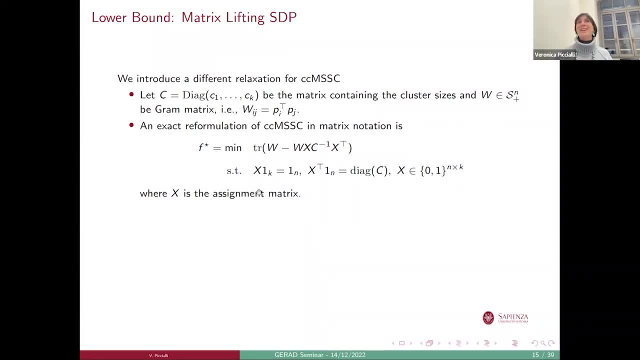 If I put the point I in the cluster J, So this is really the assignment matrix, And so what we did is to introduce a new matrix, variable Z, that shares somehow the structures of the one we had in the pangway relaxation And this we would like that to be exactly this product matrix. 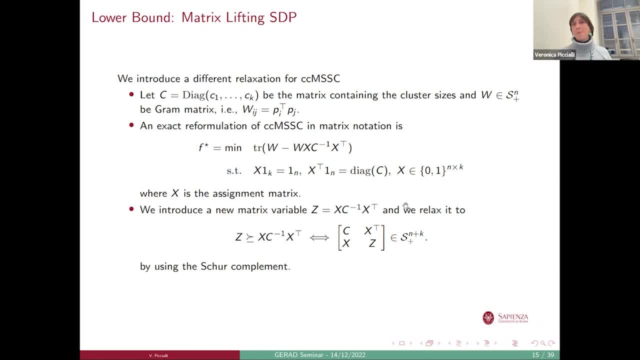 So X times C to the minus one times X transpose. But of course we relax this constraint to being this matrix being positive semi-definite And with the Schur complement We can just take this big matrix and say that this has to be positive semi-definite. 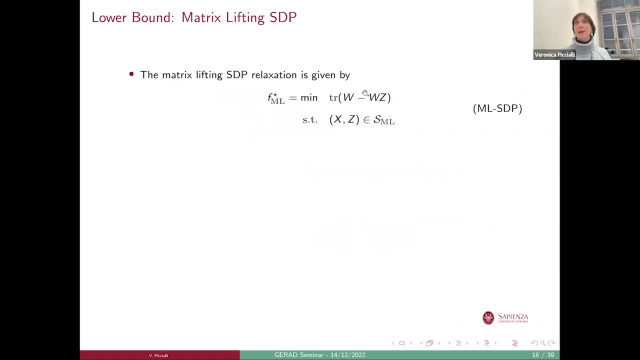 So our relaxation, then, is obtained in this way, by setting these metrics with these relaxed constraints, But our convex set, what is really relevant here, is this constraint. You see here where I'm linking the Z and the X. So this is something that allows me to keep the information on the cardinalities and to connect somehow the elements of Z with the element of C. 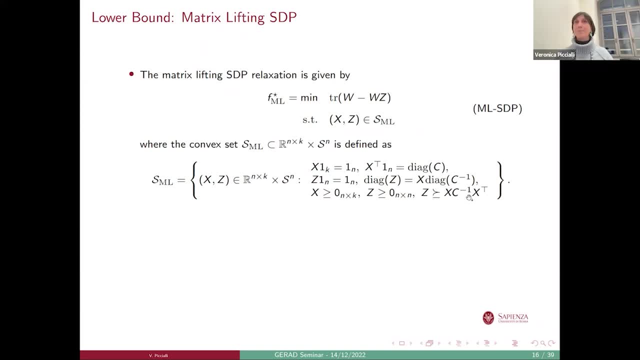 Of the of X, And so here I'm just imposing that each point has to be exactly in one cluster. Here I'm posing the cardinality constraint And here I'm exploiting the structure of Z. So what happens here? that now I only have one matrix variable of size and plus K. 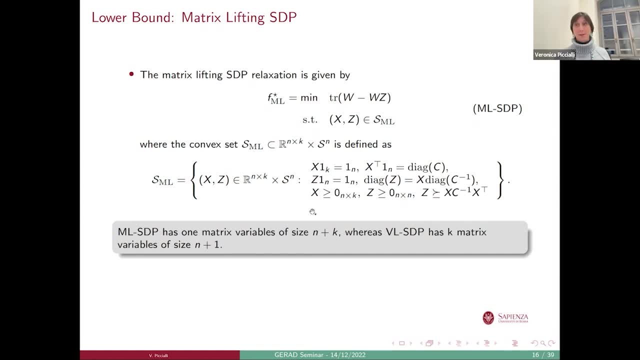 Whereas before I had K matrices of size and plus one. So when N and K grow these relaxation skills We will see in practice. also is that this relaxation skills better when N and K grow. And we can also see that this matrix Z here shares somehow the same structure that had Z in the Panguay relaxation. 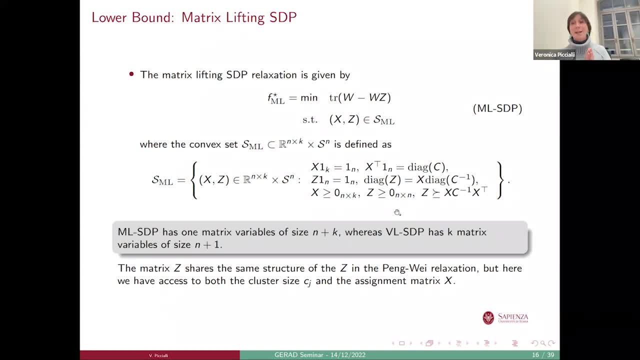 But the difference here is that now we have access both to the cardinalities of the clusters and to the assignment matrix X, Since we have explicitly the assignment, which we did not have in the Panguay relaxation. Now we are able also to impose the cardinality constraint. 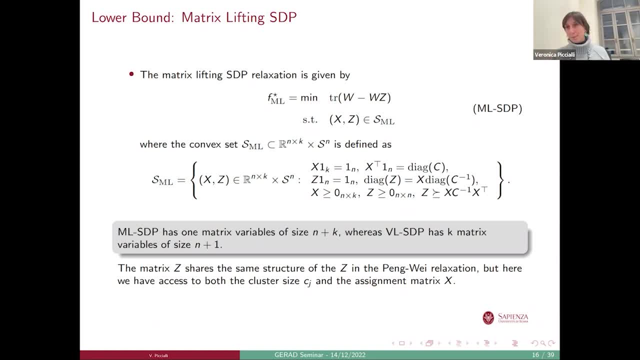 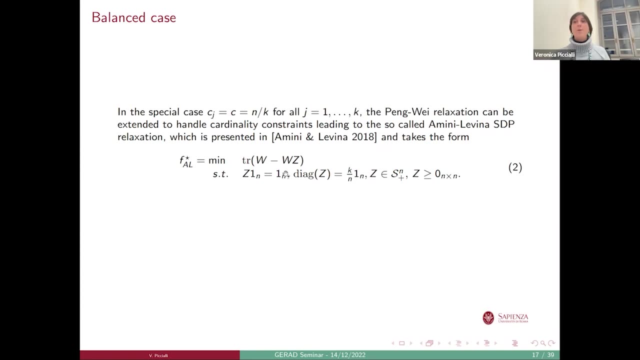 And to treat the cardinality constraints. Of course there is some price to pay because I'm still increasing the size of the matrix. I'm going from N to N plus K And this relaxation actually, if I go to the special case where the balance case, where all the clusters have the same cardinality, 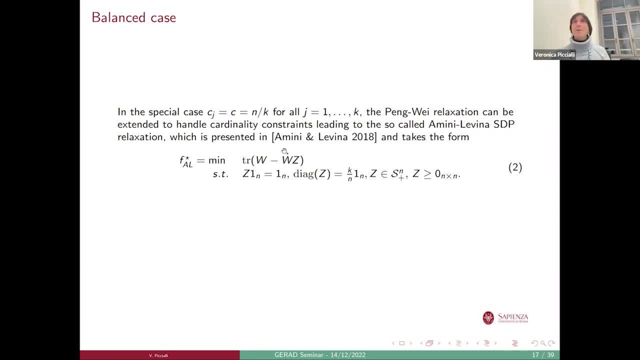 It is exactly the same as another one that has been proposed by Amini and Levina in 2018.. Which is the direct extension of the balance case From the Panguay relaxation to the balance case, And we can prove that our matrix 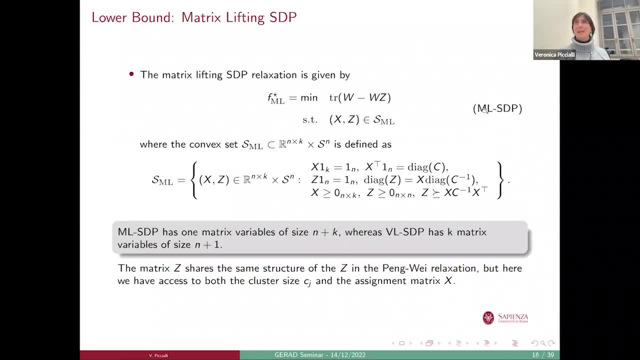 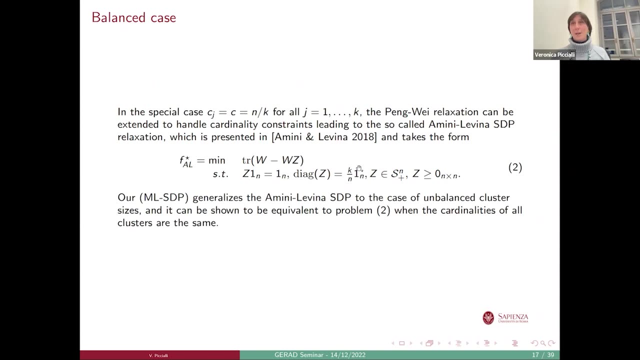 Sorry, I didn't tell you that I'm going to call this relaxation matrix lifting, SDP. So before we had, the vector lifting is the one proposed in the paper of Copt. Our relaxation is called matrix lifting, And so we can prove that our relaxation basically generalizes this relaxation to the case where the clusters have not all the same cardinality. 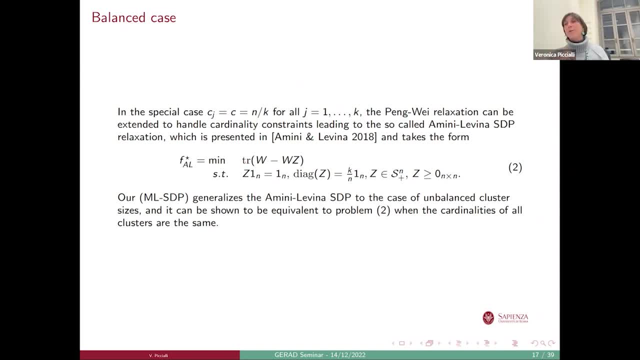 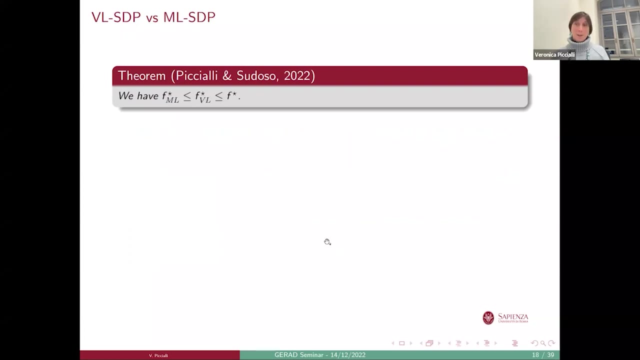 And when. If we get to the balance case, So if all the cardinalities are the same, then we end back in the Amini-Levina relaxation. So we are really generalizing that relaxation And of course one could wonder which relaxation is better, the vector lifting or the matrix lifting. 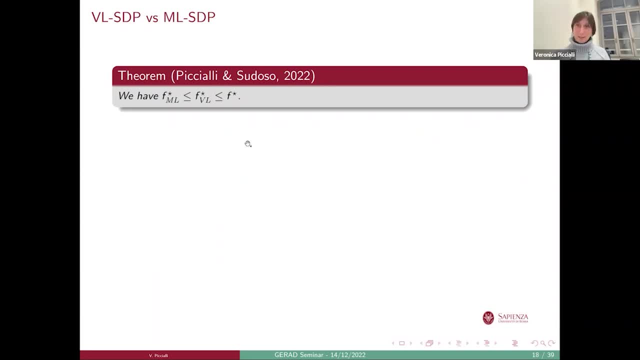 Well, and we can prove that in general, the vector lifting relaxation is stronger, So our relaxation is lower or equal. The objective function is lower or equal than the one found by the vector Lifting, So there is some place, to some price, to pay for our reduction in size. 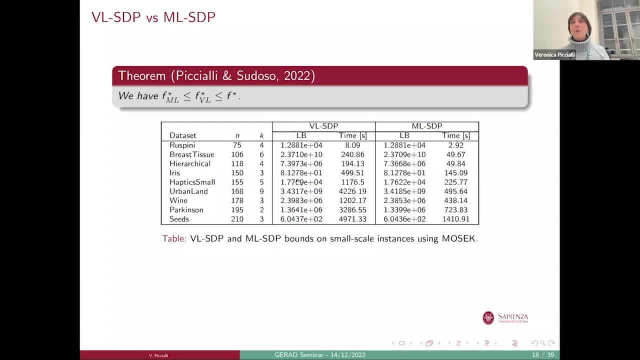 And this is something that you can see also in practice. On this table we have taken some small scale instances, because you have- And here is the number of points, Here you have the number of clusters And this is the lower bound computed by solving by Mosek. 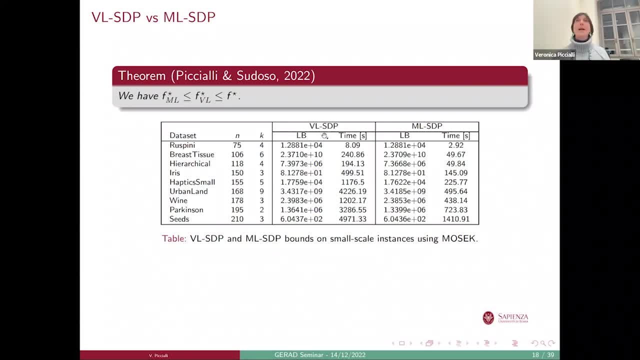 So here we are using Mosek interior point methods, Here we are solving the vector lifting, Here we are solving the matrix lifting. As you can see, the timing is always the same, So it's smaller when you solve the matrix lifting. SDP. 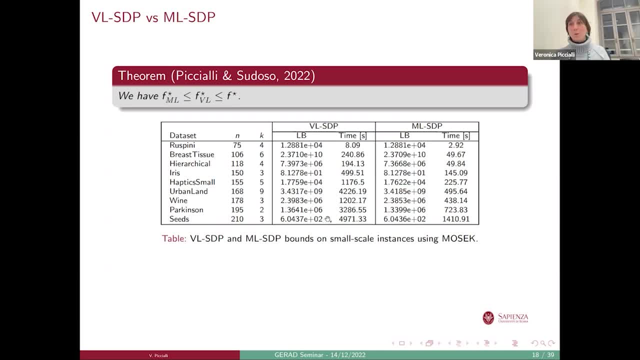 But the bound is slightly worse, Not that worse, but it's slightly worse in general. So the theory is reflected also by the computational part. However, what we want to use this, We want to use this problem inside a branch and bound. 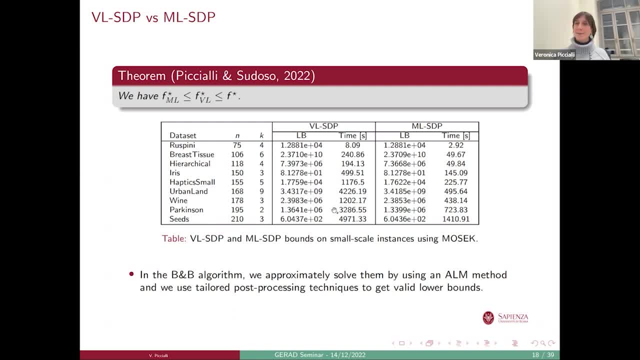 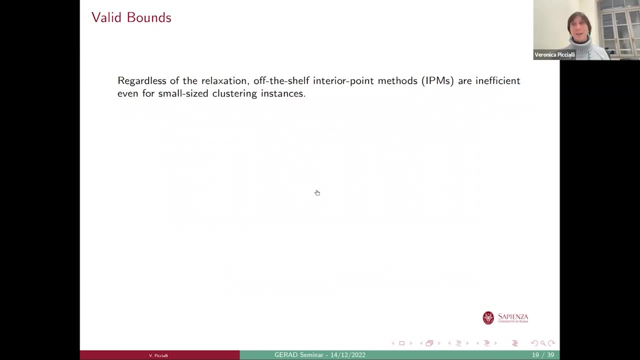 And if you look at these timings, these timings are scary, So you could never use this time for solving one single bounding problem In a branch and bound. So what we did is that we decided that off-the-shelf interior point methods were not efficient enough for solving our clustering instances. 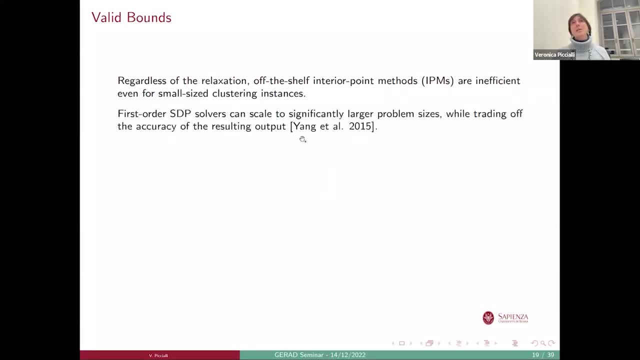 our relaxation problems. So we used some first-order SDP solvers And it is known that they can scale to significantly larger problem sizes. But there's a price- inaccuracy- to pay. So what happens when I use a first-order method that it is hard to reach high precision in a limited amount of time? 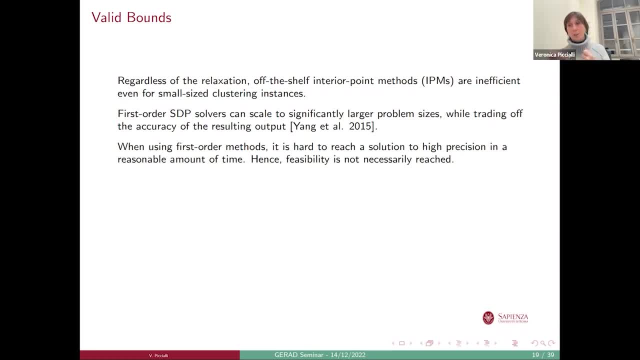 So I have to trade off between computational time and quality of the solution. So I'm going to. What we used as an accuracy for solving our SDP was 10 to the minus 4, which is a low accuracy. So this implies that in some cases we did not. 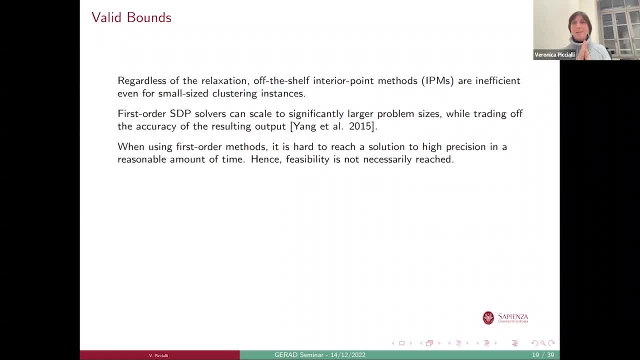 So we don't have a perfectly feasible solution. So if I'm using Mosaic, I can rely on the bound I'm getting, But if I'm using a first-order method I cannot. So what I have to do is I have to take care that I really get a safe bound. 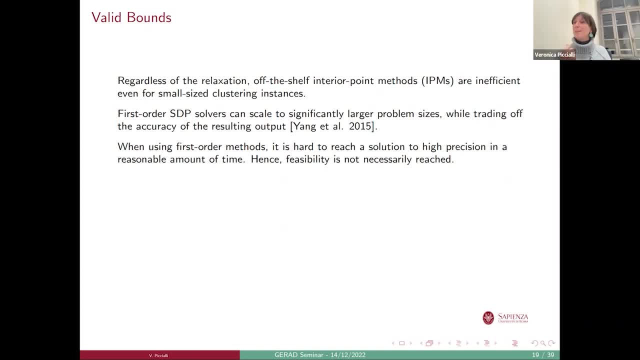 So I need some post-processing technique, because otherwise the risk is that I'm going to prune some nodes that I shouldn't. So what we did is, following the recent literature, is to use two different ideas of post-processing in order to be sure that we were generating some safe lower bounds for our SDP. 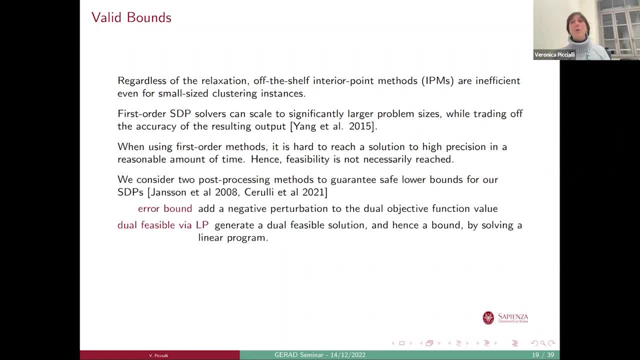 And this took In the first technique. we are basically using an accuracy. We are adding an error bound, So we are adding a negative perturbation to the dual objective function value to be sure that we are getting a safe bound. What is done in our paper is that 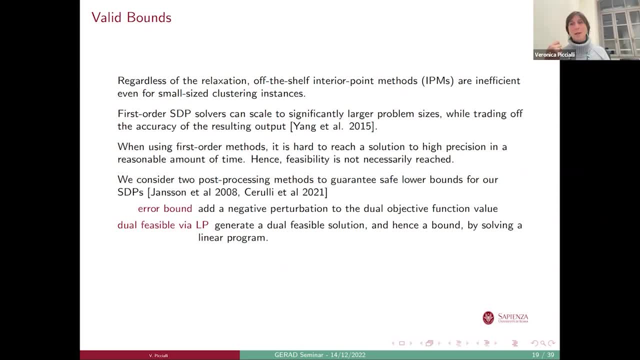 I'm not putting the details here because it requires the definition of the dual and lots of formulas, so it's not worth it. But what we did is basically to adjust these error bounds to the structure of our problem. In this way, of course, we have this post-processing phase. 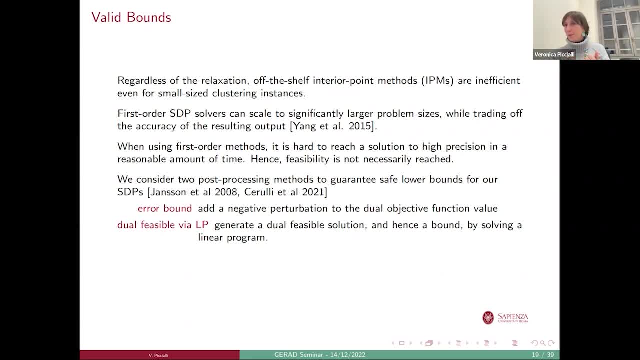 that is going to decrease the bound, So we will have a bound that is less strong than the one we would have, probably solving the problem with Mosaic, but the bound is safe and the perturbation we are adding is as small as possible. The other approach is based on LP. 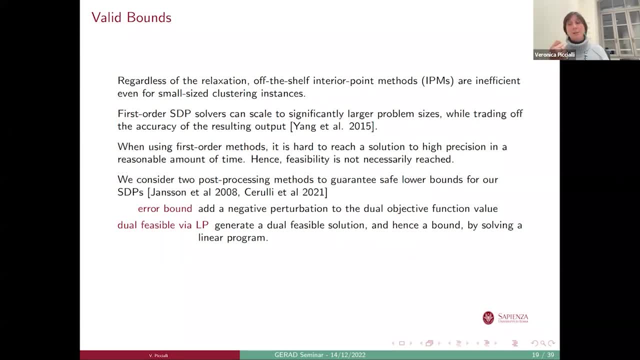 so on, linear programming, because what you do is you take the solution produced by the first-order method, you take the dual solution produced and what happens in general is that that dual solution might not be feasible because the dual multiplier variable will not be positive semidefinite. 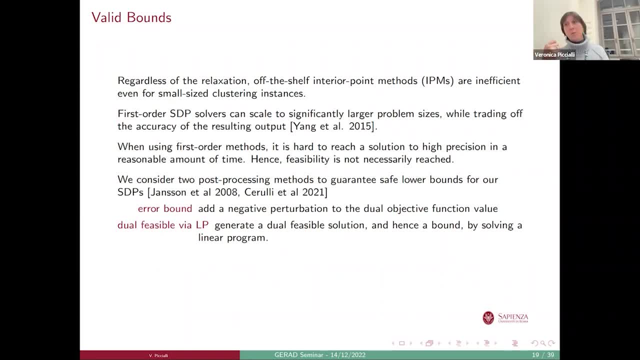 So what you do is you project that matrix to be positive, semidefinite, and by solving an LP, you try to find a dual feasible solution, And that will, of course, if it exists, provide a bound on the primal SDP. 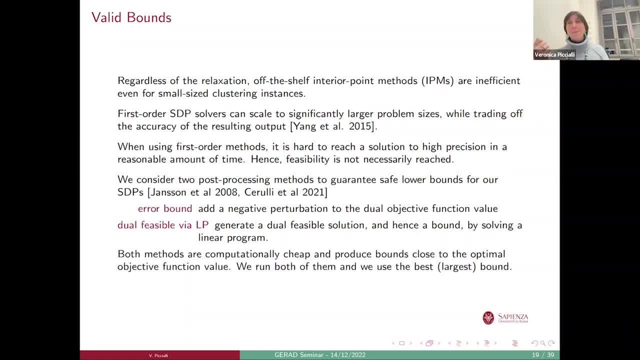 So both methods are quite cheap computationally and produced bounds that are pretty good. But we could not find a clear winner. So in some instances one bound was, in some nodes one post-processing phase was working better and in some others 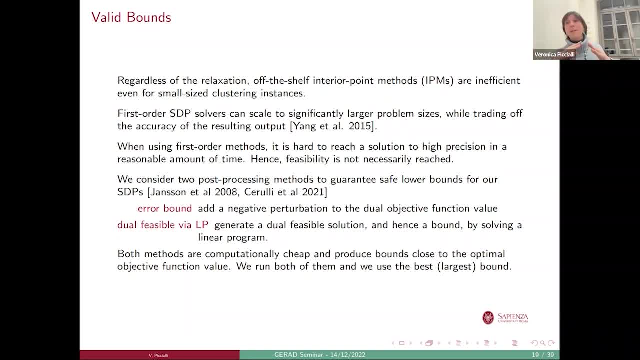 another one. what we did is, every single time we solve an SDP, we apply both the post-processing techniques and then we take the stronger bound. So we run. every time we solve an SDP, we have this post-processing phase to be sure that we get a safe bound for our SDP. 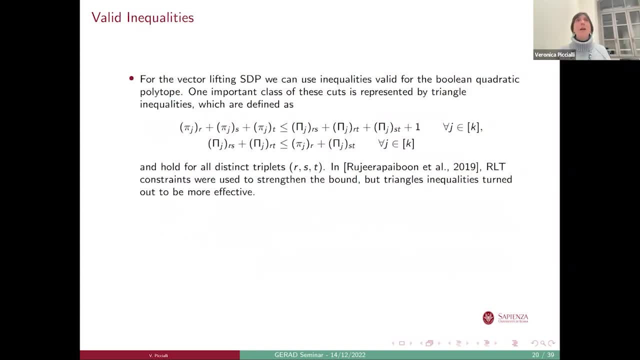 And then we get the best out of the two. So the bounds are good, but they're not good enough And, exactly as we did in the unconstrained and the pairwise constrained version, we tried to add inequalities, And this is really we will see in the numerical results. 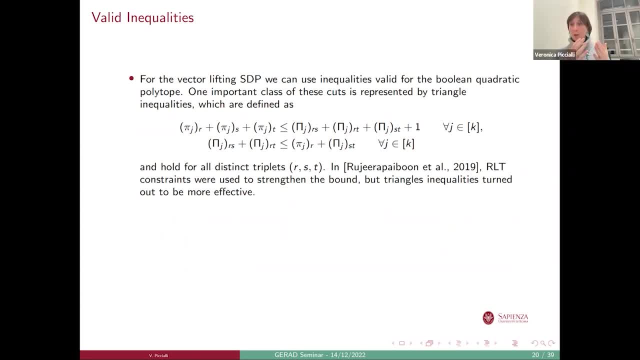 this is really a key point, So we had to choose which inequalities to add. I didn't tell you that I'm going to use both the relaxation, because the vector lifting is stronger and works extremely well when n and k are small, Whereas the matrix lifting is slightly weaker. 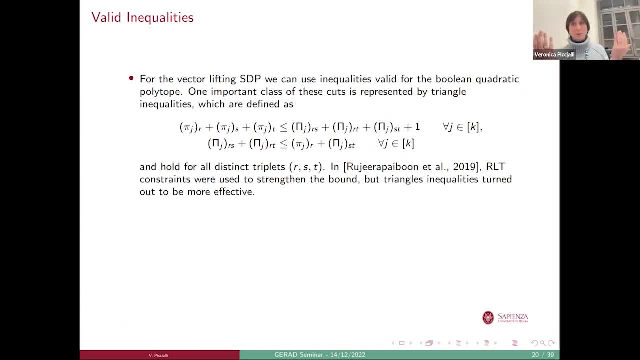 but scales much better. So what we did is we implemented two versions on our branch and bound with both the relaxation. That's why I'm duplicating everything. So I'm defining a post-processing for the mass vector lifting and the post-processing for the matrix lifting. 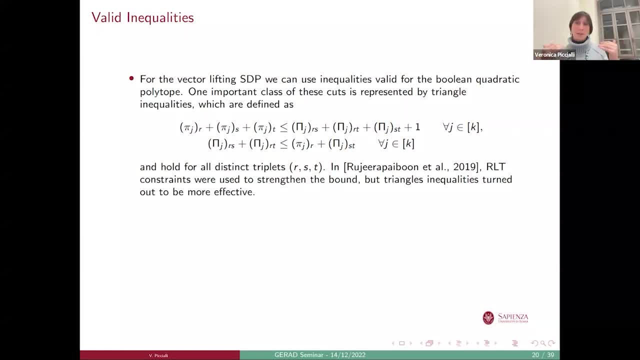 And I'm going to define valid inequalities for both problems, because I'm going to apply the same machinery of cutting plane to both problems using the proper inequalities. And actually in the original paper, where the vector lifting was defined, RLT constraints were used to strengthen the relaxation. 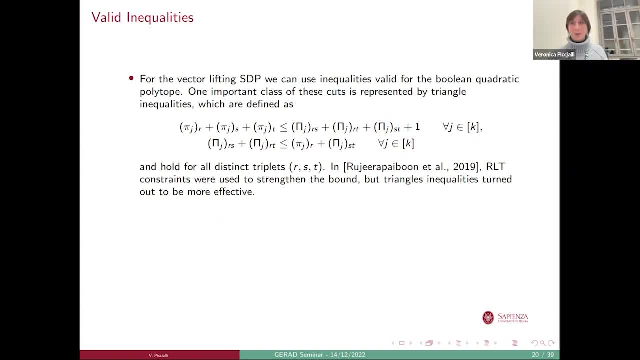 So the first thing we did was to try and use the RLT also in our relaxation. but we realized that that was expensive because there were many constraints. So it was slowing down the first order method, but the improvement in the bound was not that significant. 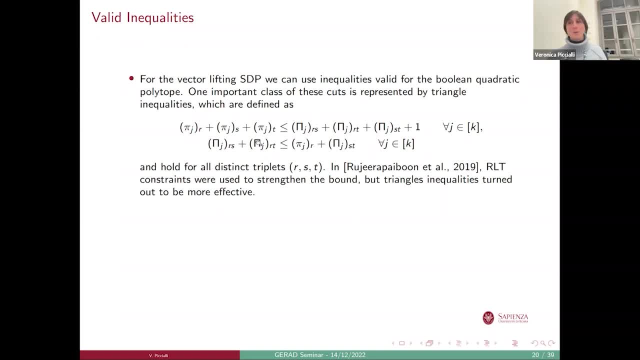 So that's why, in the end, we went back to use inequalities in the triangle inequalities, And that is much stronger. Then the bound is strengthened much more than using the RLT. And for the matrix lifting we did exactly what we did in the unconstrained and pair-constrained version. 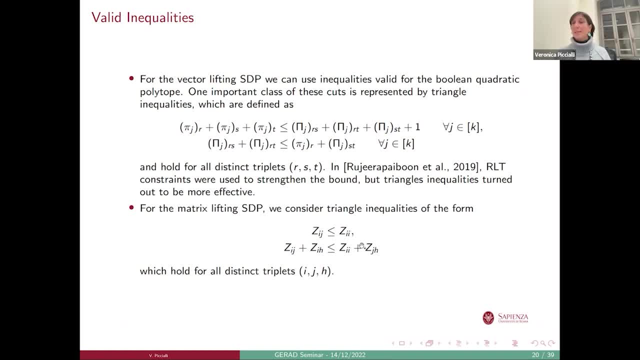 because we are adding triangles on the Z matrix, And the Z matrix, remember, resembles the structures we had in the unconstrained and pairwise constrained version. So in both cases, what we are doing is we are adding the inequalities in a cut-in-plane fashion. 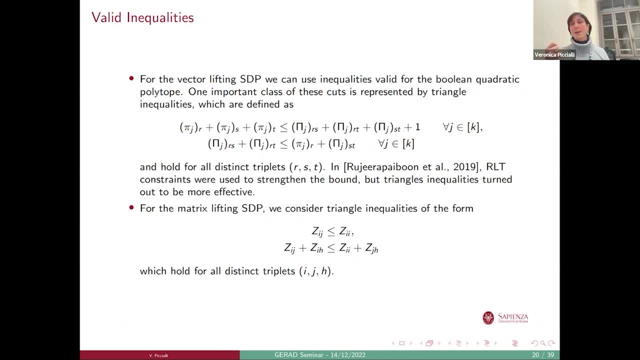 So we find like 1,000, 100,000 inequalities. We order them by violation and every cut-in-plane iteration we add 10,000 inequalities that are violated And then we remove the inactive ones. And also I should mention that we inherit. 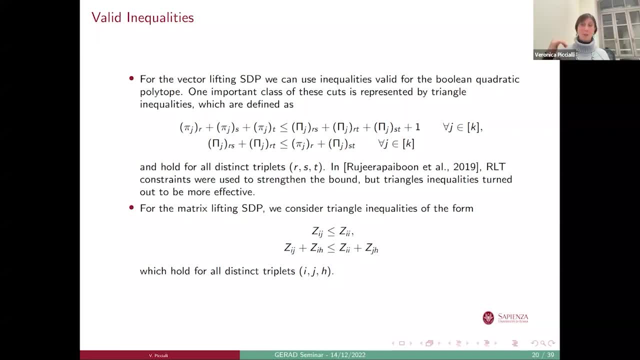 from the father to the children, the inequalities, because we have seen that this is much more effective than recomputing the inequalities. So this is what we do for the lower bound. As for the branching strategy, the most natural branching strategy here would be, in some sense. 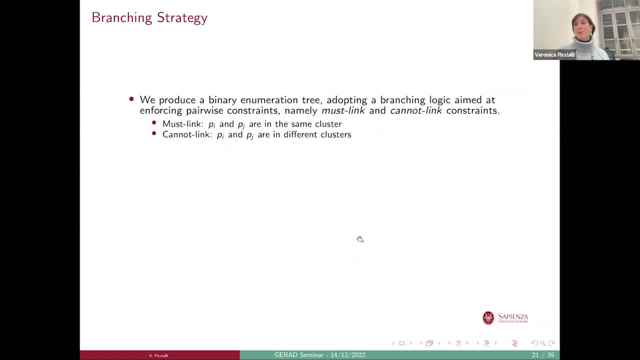 to take, you know, the assignment matrix. We have the assignment matrix both in the vector lifting and in the matrix lifting, And then we can say, okay, I take the component of that matrix that is more far away from me, And then we can say: 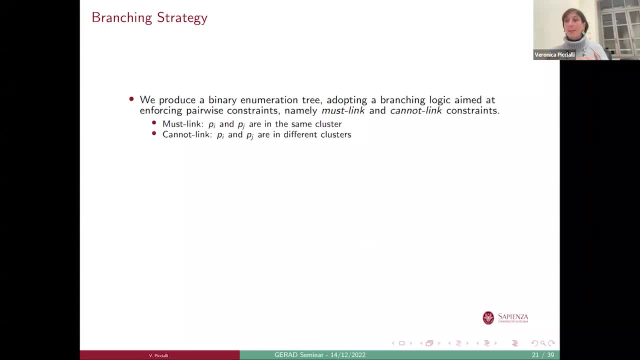 okay, I take the component of that matrix that is more far away from me, And then we can say: okay, I take the component of that matrix that is more far away from me, and then I'm going to fix that one to zero in one child. 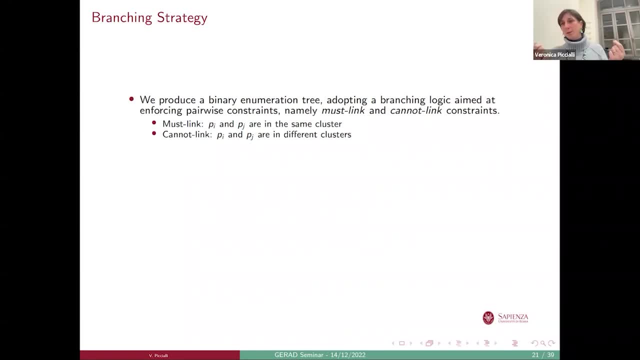 and to one in the other, And then I'm going to fix that one to zero in one child and to one in the other. So this could be the most straightforward choice, But then we decided that we stuck with the pairwise branching. So what we do. 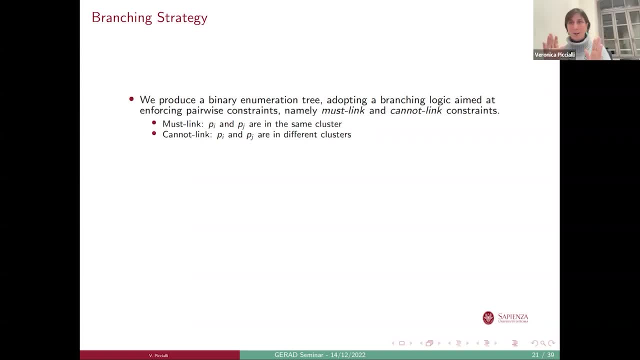 is, we take a pair of points, The one where we cannot decide which one I'm using. It doesn't matter whether they are together or they are not produce on one child. we decide that those two points will be together, and on the other we 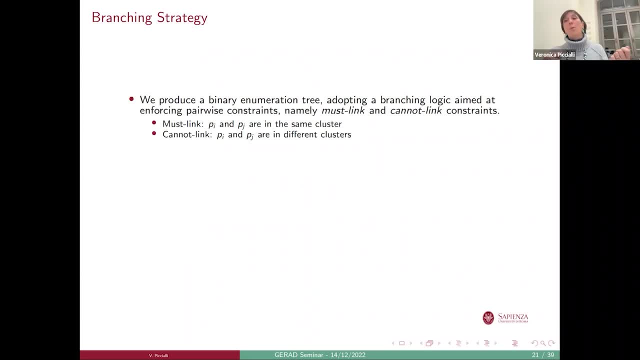 decide that the two points will be separated. So on the one child we put the mass-linked constraints and on the other child we put the cannot-linked constraints. Also, in this case we will see that for both relaxation this translates into adding some linear inequalities in the children. so we can 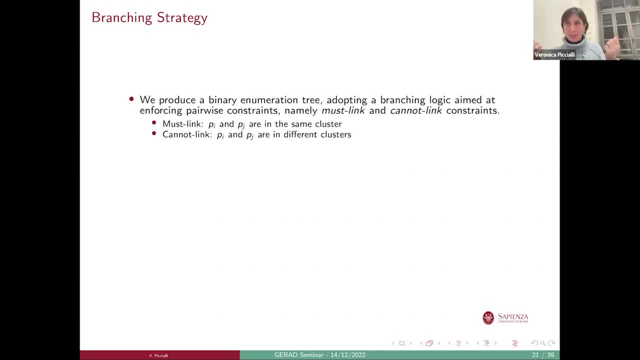 easily enforce the pairwise constraints, exactly as we did in the other two versions. So why did we prefer this one to doing the standard branching on the elements of x? Well, for three reasons. The first one is that this has somehow more impact because it allows: 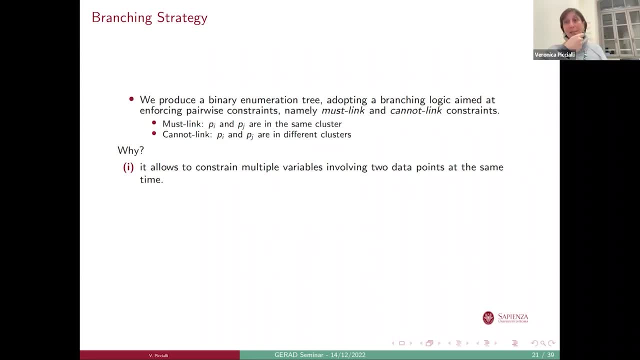 to constrain multiple variables that involve those two data points at the same time. so in general it has more effect. Also it allows to explain some symmetry reduction techniques and we will see that we can again reduce significantly the size of the SDPs that we solve. And also this implies that basically with this algorithm we 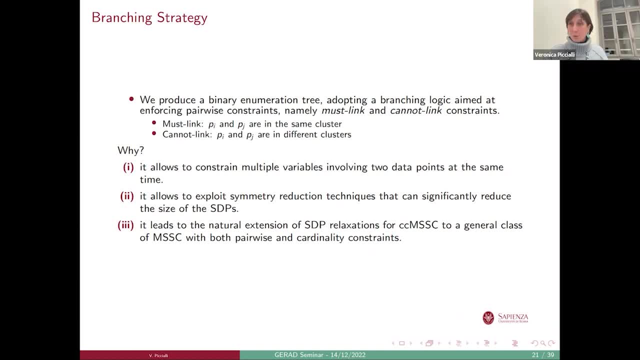 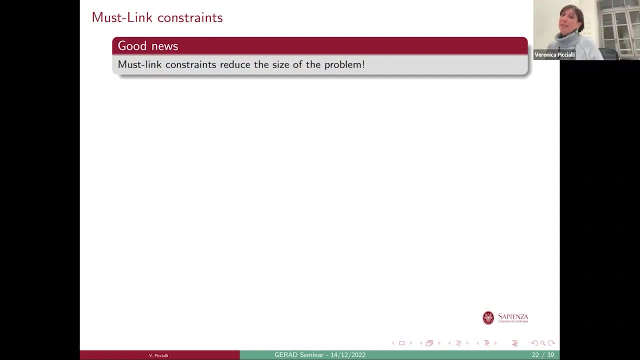 are able also to solve problems that have both pairwise constraints and cardinality constraints. So if I have both kinds of background knowledge, I can include both of them in my problem and still be able to solve it. so we can treat both types of constraints. So also in this case, the good news is that having the mass-linked constraints that are generated by 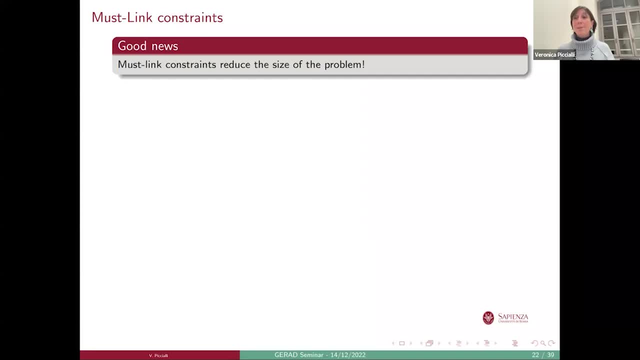 the branching decision helps us to reduce the size of the SDP. we solve Indeed if we have the mass-linked graph. so in this graph we have that the nodes are the points and we have an edge. only if there is a mass-linked constraint between those two points, then we compute the transitive closure of that. 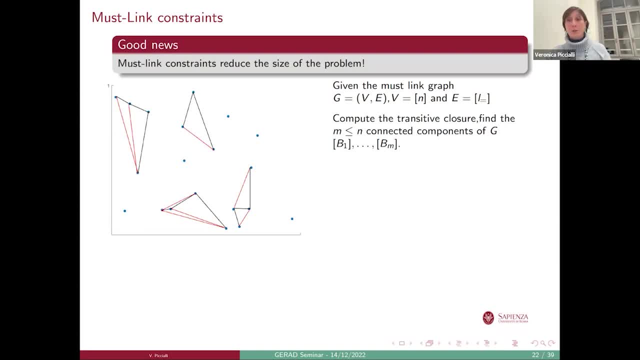 graph and find the connected points. So we can then compute the transitive closure of that graph and find the connected components, which will be m, which in general is smaller than n, And we encode this transformation. so we define a suitable transformation, matrix T that tells you whether a point i is in the connected component or not. 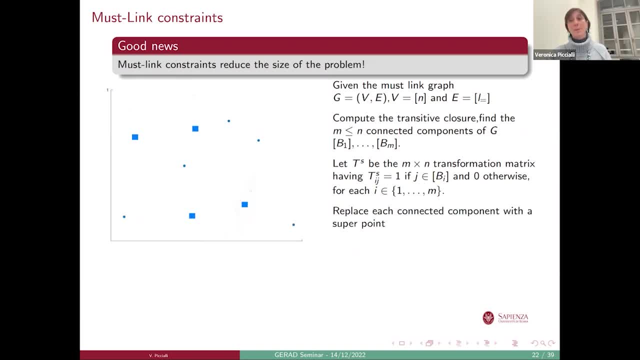 And then we replace each connected component with a superpoint, And so this basically allows us to reduce the size of all the matrices involved in the in the SDP problems, and instead of clustering the initial data point, we find the k-partition of the superpoints so a much smaller. 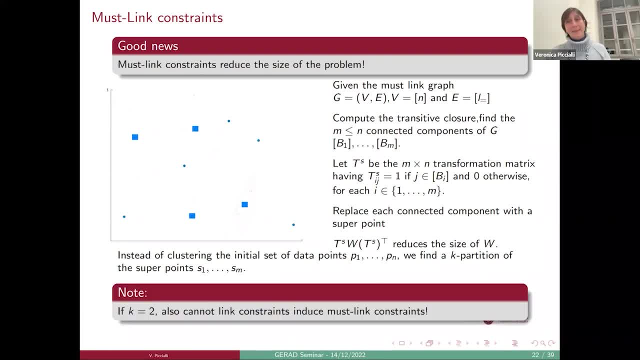 set of points. And the even better thing is that if by chance k is equal to 2, also when you have cannot-link constraints, that will enforce automatically some mass-linked constraints. So in that case this is even more effective because this allows to reduce the size more than in the in the general in. 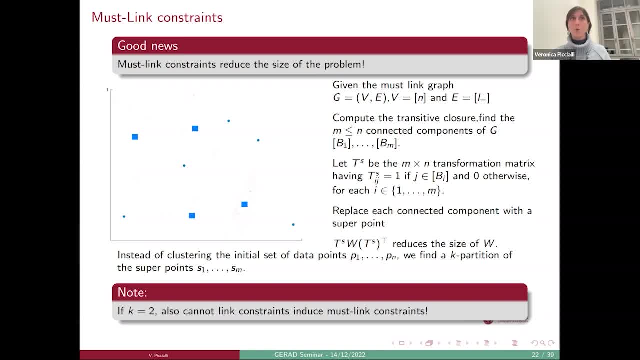 the mass-linked constraints in k-differentiated clusters. So this is even more effective because this allows to reduce the size more than in the in the general in the mass-linked constraints in k-differentiated clusters. So this is even more effective because this allows to reduce the size more than in the in the mass-linked constraints in k-differentiated clusters. 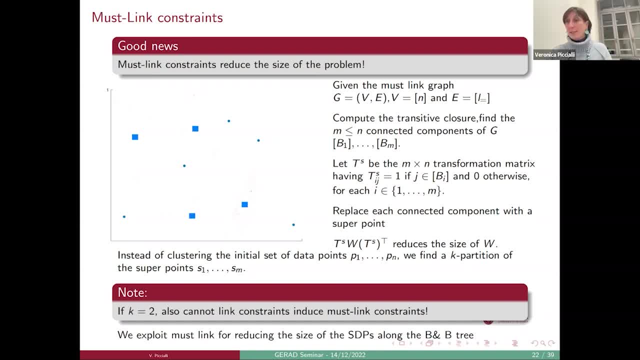 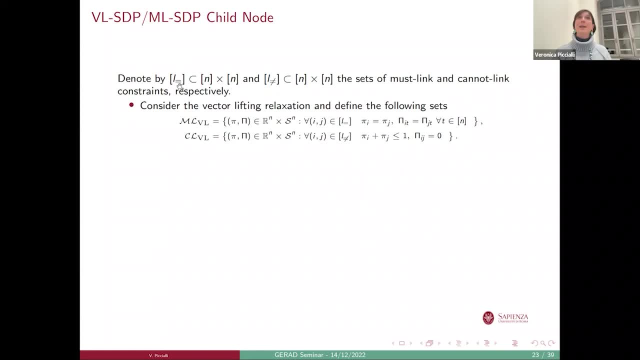 So we exploit this result to reduce the size of the SDPs along the branching boundary In particular. if I denote in this way, you see here, the set of mass-linked and the set of cannot-link constraints, I can, you see, introduce some linear constraints here in. here I'm talking. 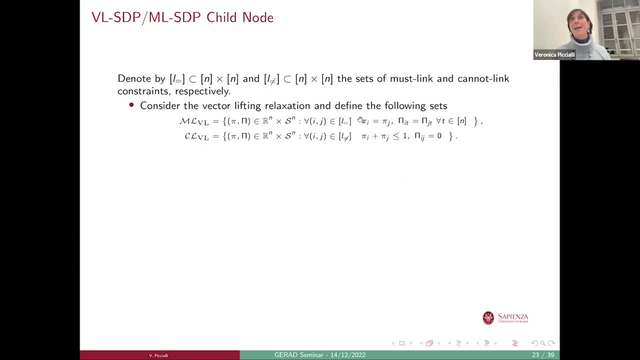 about the vector lifting formulation where, remember my pi were just the cluster indicator vectors. so I have vector length and that tells you if point i is in the, in the, in the mass-linked, and that tells you if point i is in cluster j or not and as you can see here, say a mass-linked. 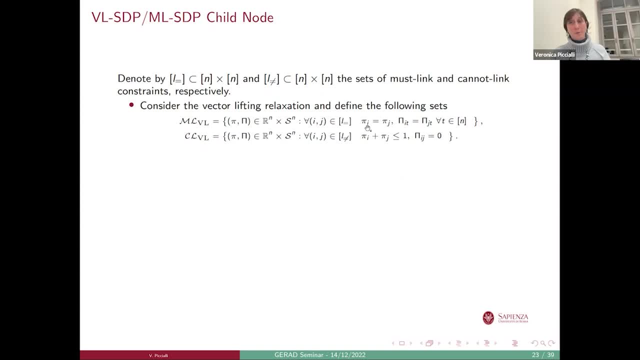 constraints implies that the two cluster indicator of for those two points will be the same and the same. this equality reflects also the matrix on capital pi. if I have a cannot-linked constraints, then I know that this two cannot be the same and at most one will be one. so this is what happens. 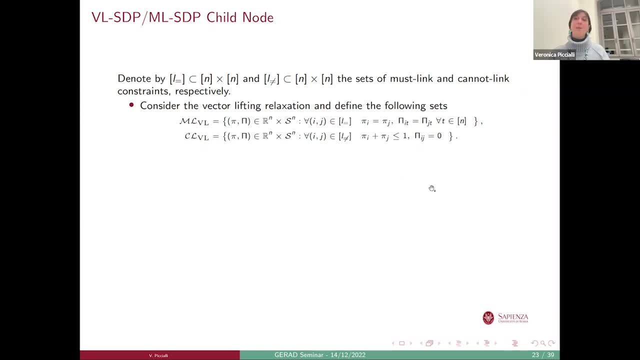 on the on the big matrix, That the elements i, j becomes equal to zero. so again I have linear constraints and the same thing is both as reflects on linear constraints in the matrix, lifting both on x and on z. so you see, if I have a mass-linked constraints, then the two rows i and j of z need to be equal. 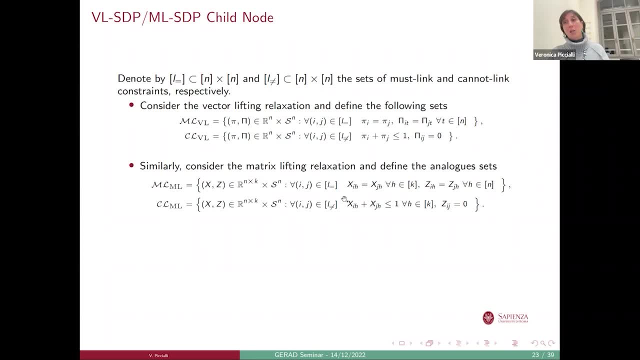 and also the elements of the assignment matrix of i and j need to be the same and if I have a cannot-linked constraints, this translates into these two linear constraints. so you see, I can easily encode by linear inequalities the mass-linked or cannot-linked constraints. however, that's not. 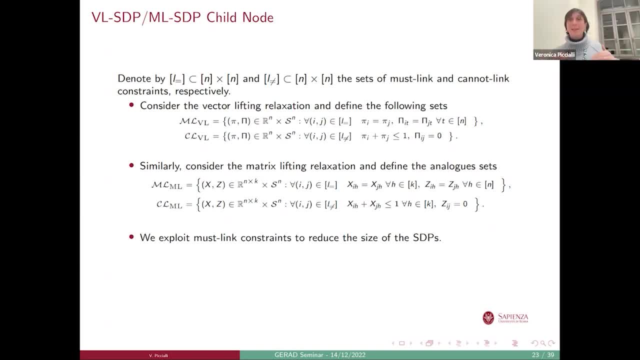 that's not what I want to do. I don't want just to throw inside the linear constraints and solve again the SDP in the children. what I want to do is really reduce the size of the SDP again, and this can be done by introducing some suitable transformation. so what happens in? 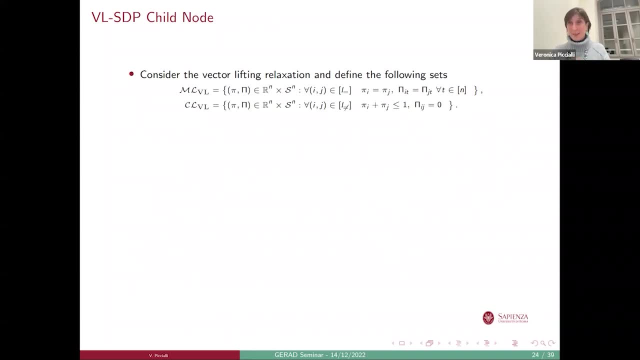 the vector lifting child node on the mass-linked side. so when I'm adding a mass-linked constraints- because only mass-linked in general allow me to reduce the size- is that this was my original problem, where I have a certain number of variables related to the number of points I'm considering in that node, and then I can define an equivalent problem. this is exactly. 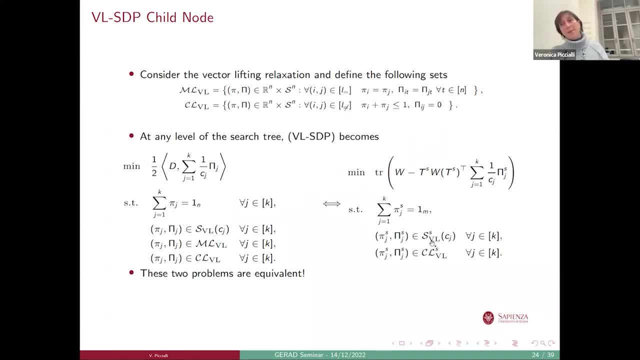 the same problem, but on a smaller positive semi-definite cone. and this how smaller? well, that depends on the number of connect components. this s is basically the number of connected components that I'm finding in the graph of the mass-linked constraints. and these two problems are: 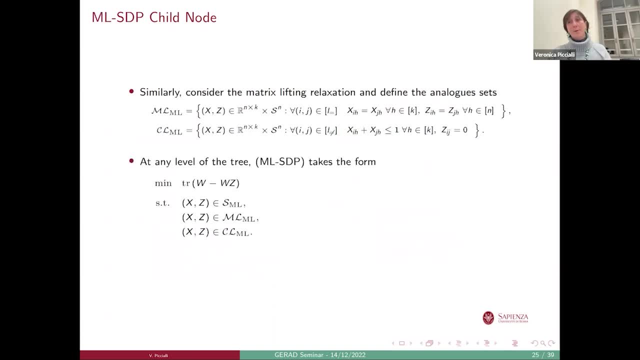 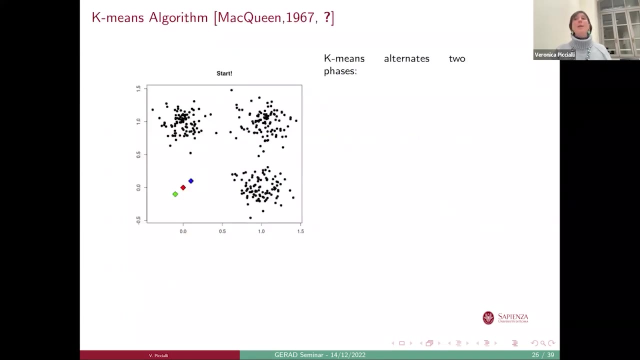 perfectly equivalent And the same thing. I can prove it in the matrix lifting relaxation. so again I'm solving a problem that has the same structure, but now all the matrices are smaller, so I'm working on really smaller positive, semi-definite cones. What about the heuristic? so now I told you about the branching. 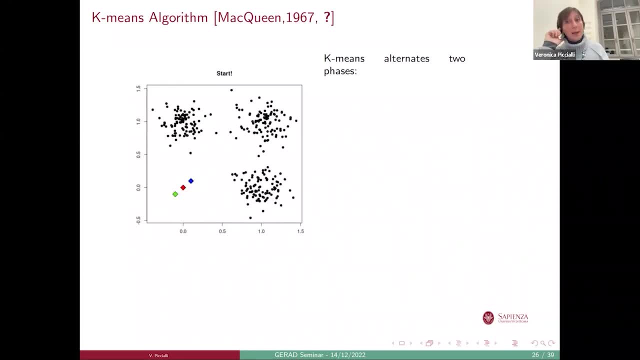 I told you about the lower bound. I still have to tell you how we compute an upper bound. The most famous heuristic for unconstrained sum of square, minimum sum of squares, clustering, is K-means, And K-means alternates. basically two phases. the first one is the optimal assignment of the points. 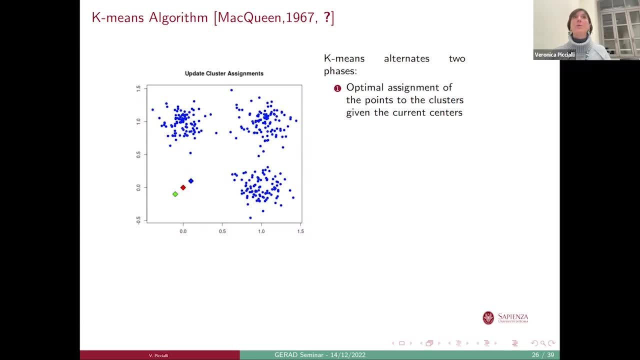 to the cluster once I know the current center. so if this is the situation, you see, these are the three centers and this is the optimal assignment given these three centers. Then I move again the centers given the assignment I've just done and I iterate between these two phases, you see, and 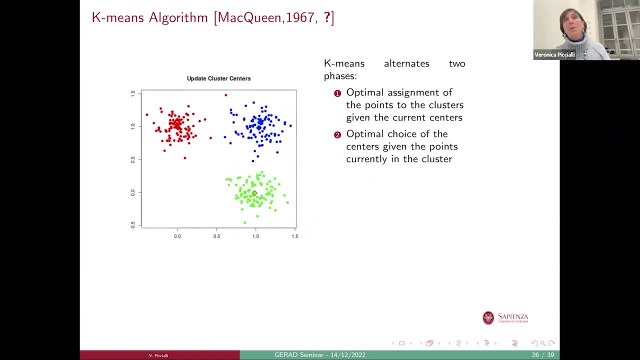 what happens is that I will stop when, basically, the centers stop moving, So when the solution does not change anymore, that then I stop and what I get is a suboptimal solution that heavily depends on the choice of the centers, on the initial choice. So what happens? 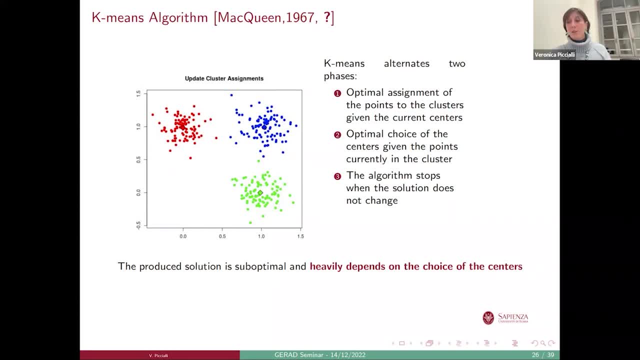 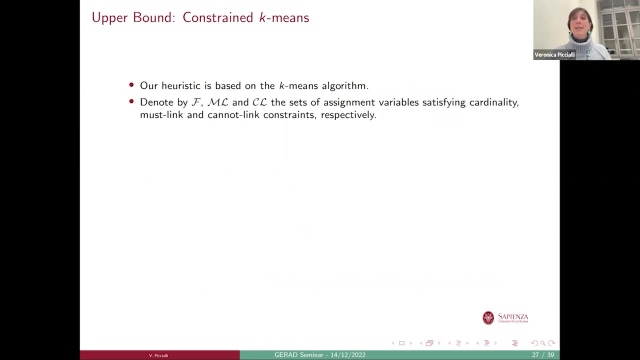 here, however, is that I cannot. in the original version of K-means, I do not have constraints, so I cannot include either pairwise constraints or cardinality constraints, so what we need is a constrained version, But what we do is basically something similar. What we do is again to alternate two phases: one for selecting the assignment and one for selecting. 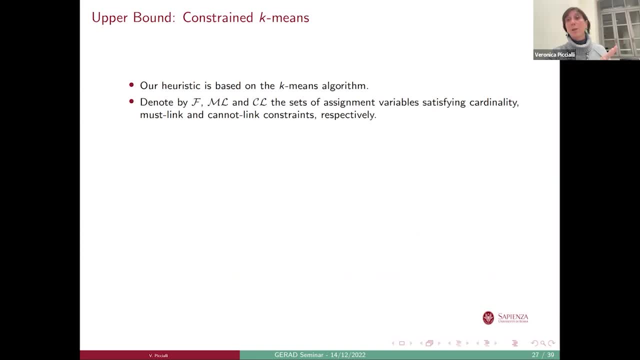 the centers. but in doing so we keep into account all the constraints we have, because we run the heuristic at each node of the tree. so we may have some must link and cannot link constraints that derive from the branching decision and, of course, the cardinality constraints. So this is what 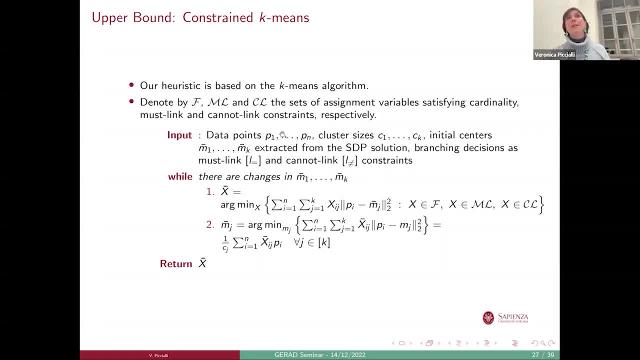 our algorithm works. we have, you see, the data points, cluster size, and then we have some initial centers. that will tell you in the next slide how we extract from the SDP solution. and then we have the must link and cannot link constraints. then we have the current node And then what we do here: we just solve an assignment problem and this is. 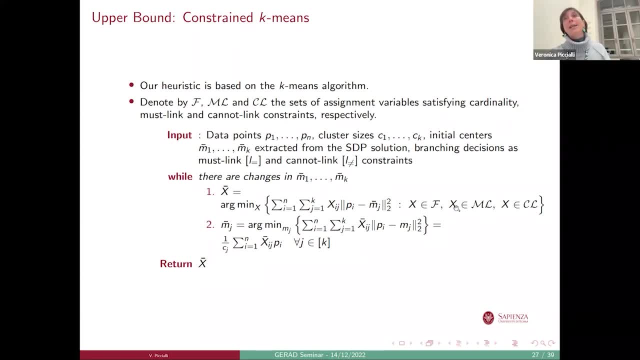 an integer linear programming problem where we are trying to solve our problem for the fixed centers. So this is an integer linear programming problem where we are encoding in the assignment matrix the cardinality constraints, the must link and the cannot link constraints. So this is a feasible clustering and Gurobi solves this problem in zero time. 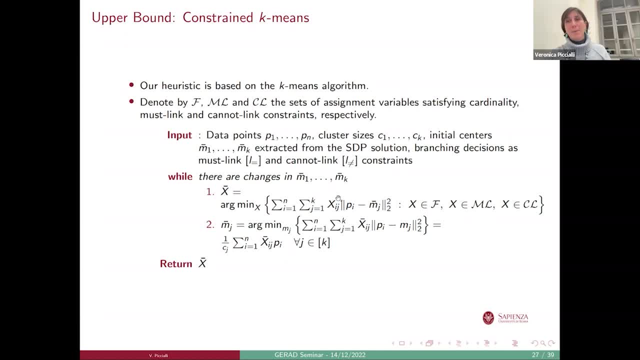 basically with no difficulty for fixed value of the centers. the problem for Gurobi is extremely easy. And then, once we have the assignment, we just compute the centers in the usual way, so that is the barycenter of the points in each cluster, and we iterate until the centers do not move anymore. 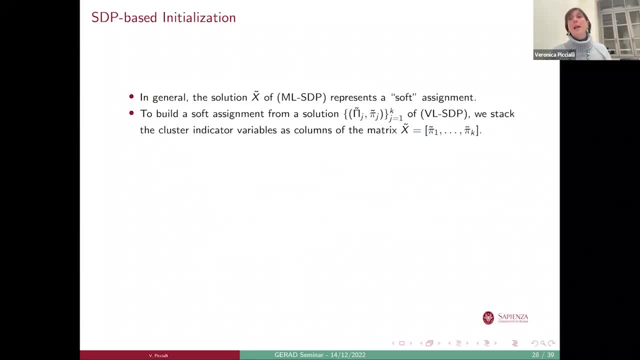 How do we choose the initial set of centers? Well, if you think about our SDP relaxation, what you get- we get in output in general- is not the real matrix assignment, but it's a soft assignments because we are not imposing binarity of the variables. so what happens is that we will have some elements of x or pi. 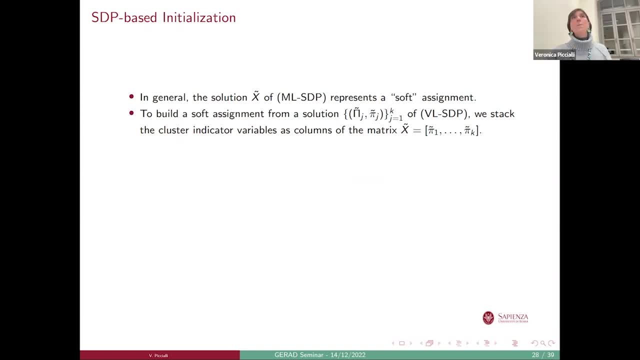 that are between 0 and 1.. So what we do is we try to build a hard assignment, so a real assignment that is as close as possible, in terms of Frobenius norm, from the soft assignment by our SDP relaxation. And we do so again by solving an integer linear programming problem. 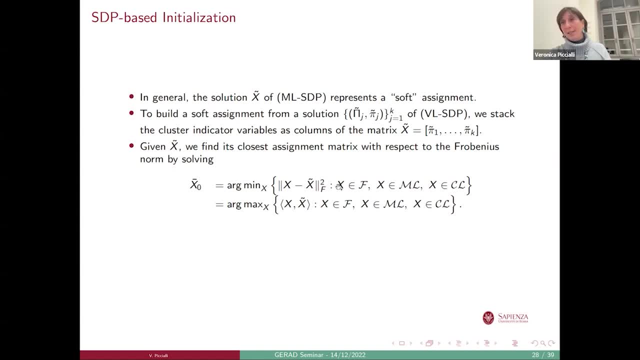 where, sorry, quadratic- in this case a convex quadratic integer programming problem, And again, this is solved extremely fast by Gurobi. so we use Gurobi for solving this problem, And so what we get here is: you can actually not, sorry, you can rewrite it as a linear. 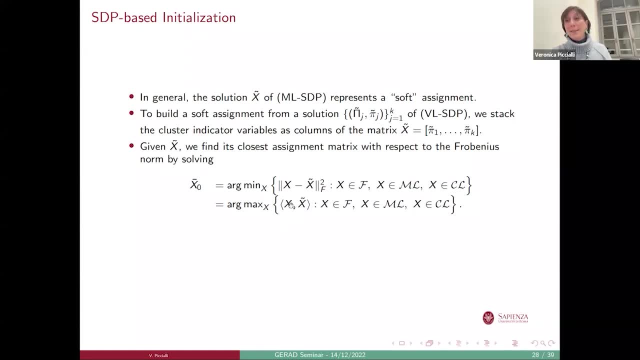 integer linear programming problem. And so what we get, you get here is the hardest that mostly resembles, that is feasible and mostly resembles the solution of our SDP. So again you see that we are relying on the quality of the SDP solution. So the better the solution, the better will be this initial choice of centers, because once we have the assignment, 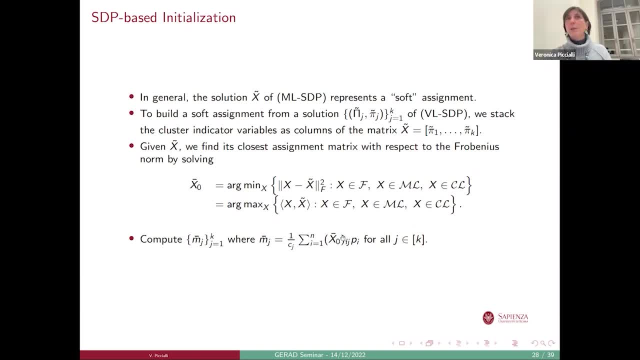 again, we derive the center in the usual way. So we know that for a given assignment, the optimal center is just the body centers of the cluster. So that's what you get. OK, now that I gave you all the details, I can tell you what are the numerical results. 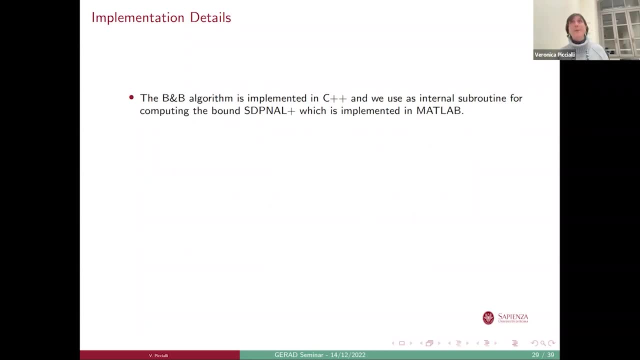 So our algorithm is implemented in C++ and we use as internal subroutine for solving all the LTPs SDPnL and SDPnL+- sorry, SDPnL+- which is implemented in MATLAB, And we use Gurobi for solving all the integer linear programming problem that we have in the heuristic phase and also for solving the linear 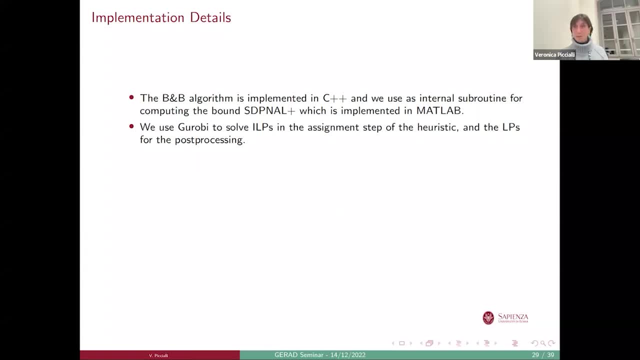 programming problems that come from the post-processing phase for getting safe bounds. The machine where we run the experiment is a laptop, a powerful one, which is a gamer laptop. So it's a powerful one, but it's just a laptop And we implement two versions. 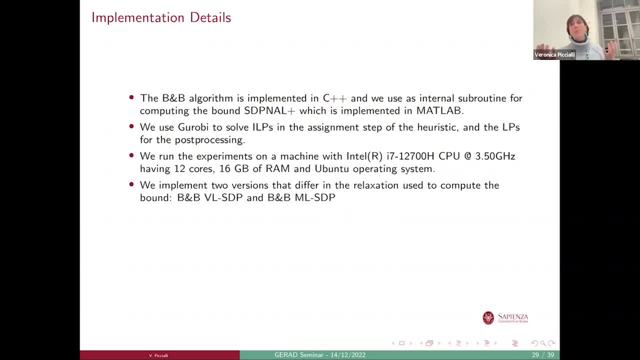 as I told you of our branch and bound, because we really want to evaluate in practice the quality of the tools in relaxation, the vector lifting and the matrix lifting. So the only difference is the relaxation that we are using for computing the SDP bound. 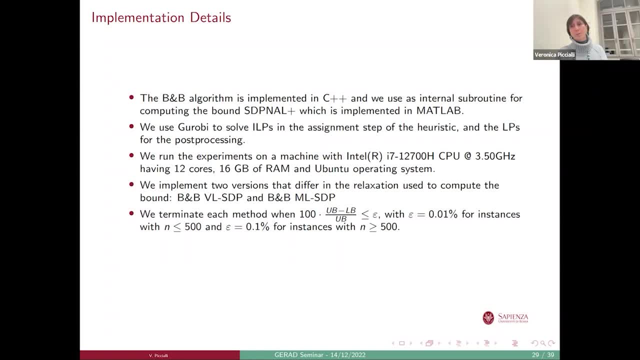 And for the stopping criterion. we have two different stopping criterion depending on the size of the instances. So we have the 0.01% on the optimality gap for instances smaller than 500 nodes, whereas we have 0.1% for instances with then larger than 500. 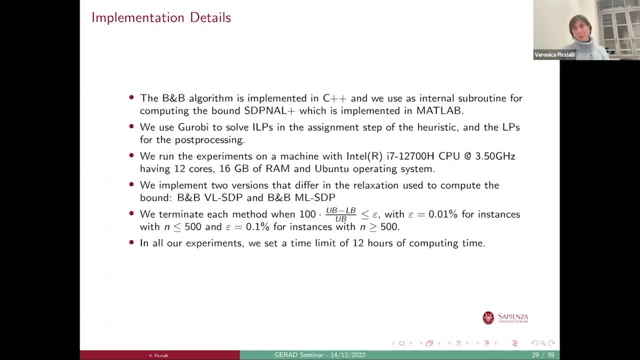 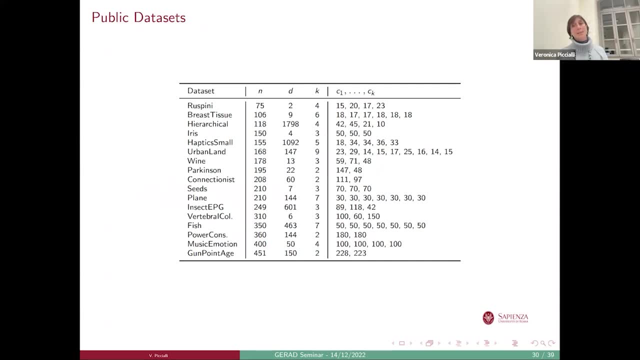 And we have a time limit of 12 hours computing time. So here are the instances we are solving and these instances are all real world data set. They basically come from classification problems. So we are using a number of clusters, the number of classes, because we know the ground truth here. 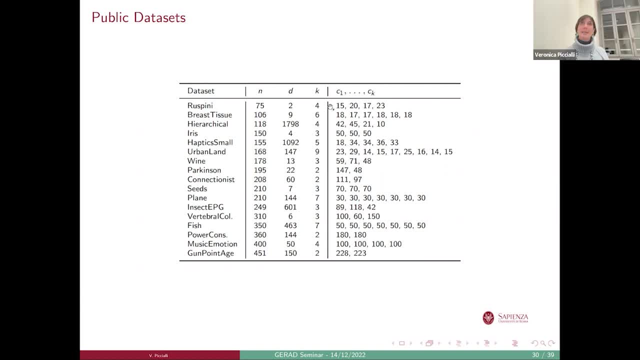 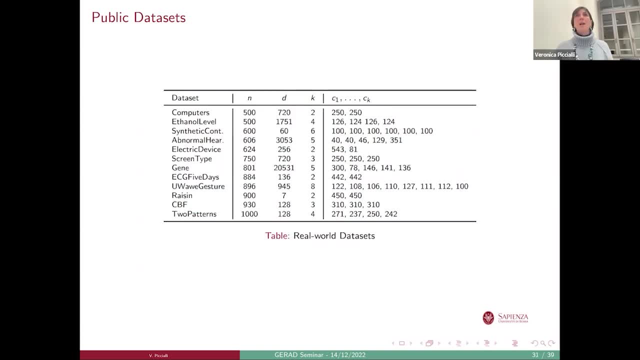 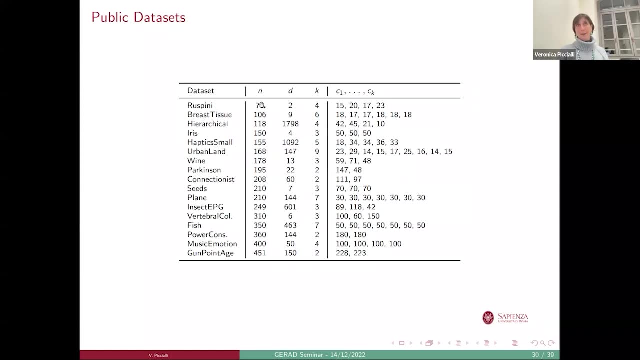 Most of them are with the different cluster sides And here are the larger ones. So you can see that we go if you look at the sides. we go from n equal to 75 for the Ruspini instances, which is in the plane, to instances with 1,000 points. 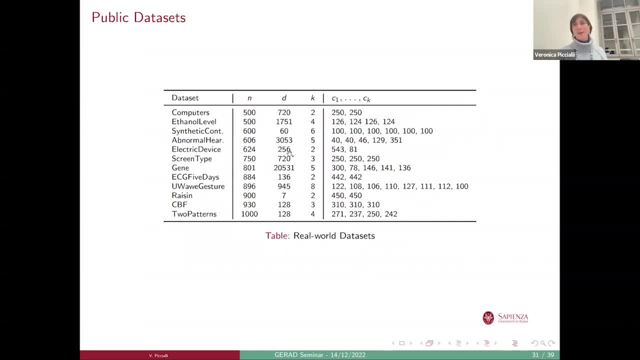 And also the number of fissure is extremely variable, And this does not affect at all our problem, because we don't see it in our formulation, So we don't see the d. So the d can be anything You can see here. there is also 20,000.. 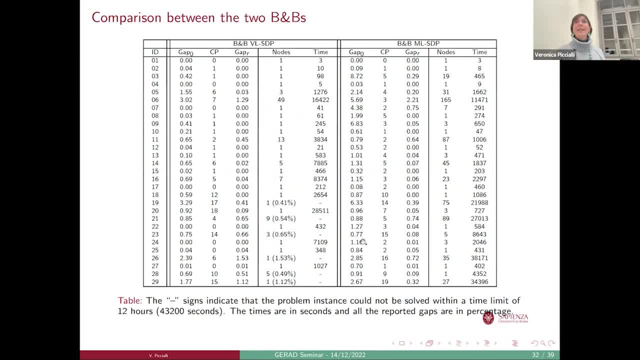 So that is not an issue. And here is the table of results. But we just compare the two branch and bound, The one where we use the vector lifting and the one where we use the matrix lifting. I don't want you to look at details at the table, but just to give you an idea of what I'm representing. 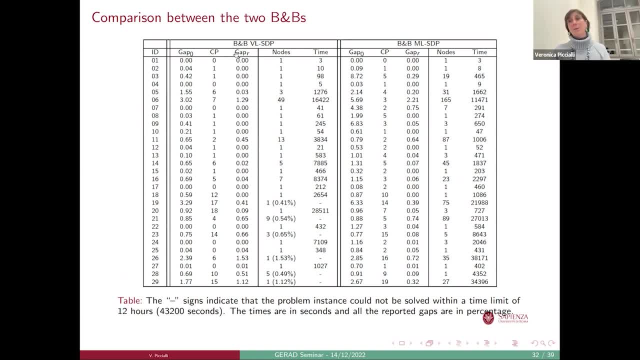 So these first three columns represent the behavior at the root node. So this gap zero is the gap that you reach after you do no cut in plane iteration. So you are just solving the pure SDP relaxation. On this column I'm solving the vector lifting SDP. 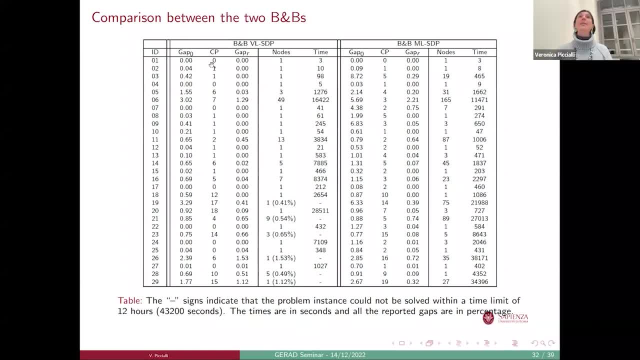 On this column I'm solving the matrix, lifting SDP. Here is the number of cut in planes I'm performing, because I stopped the cut in plane if I don't find violated inequality, So if the bound does not improve enough. And here is the gap at the end of the root node. 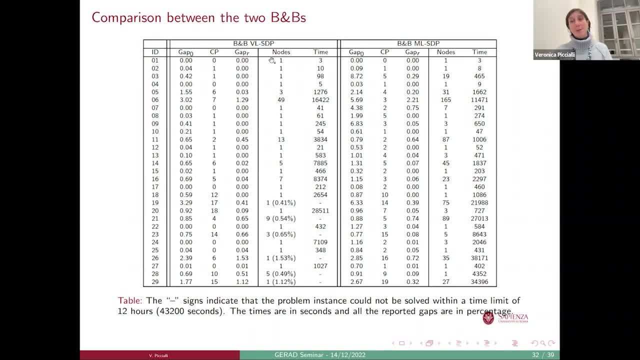 And then here, on these other two columns, I have the final number of nodes that are needed for solving the distance and the time needed. And you can see that in some cases, here you have this sign, this minus sign. In that case, in 12 hours the algorithm did fail in solving to global optimality and closing the gap. 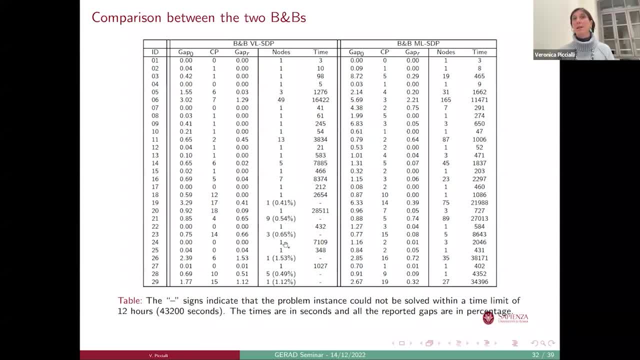 And so you see here in brackets, you see here the percentage gap when the algorithm stopped. So this left side is for the vector lifting SDP, This right side is for the matrix lifting SDP, And all the timings are, All the times are in seconds and all the gaps are in percentage. 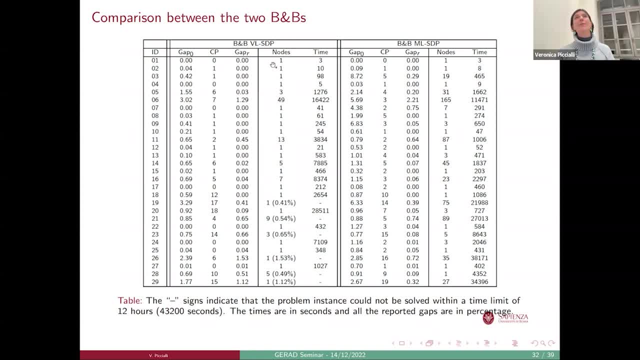 So what happens here says that if you look at the first part of the table and the instances are ordered in increasing size, So the first instances are the smallest, the one with the smaller number of points, And then, when you go down, the size of the instances is growing. 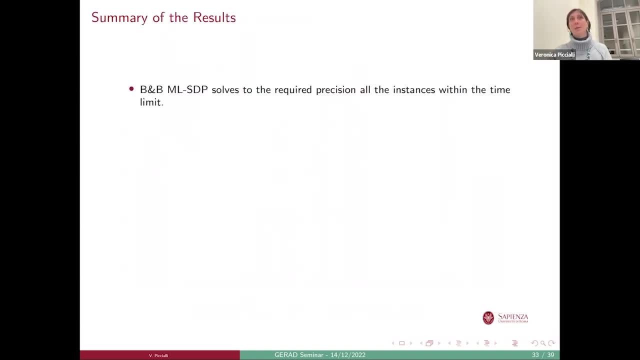 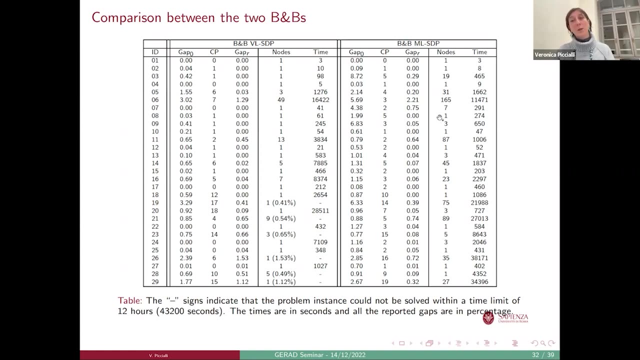 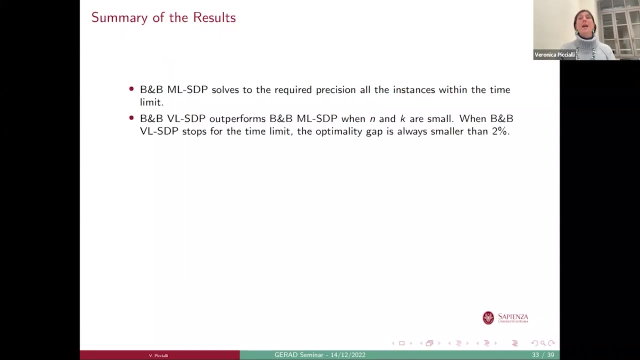 And while the conclusion that you can draw are these ones, like, as you can see on this side, there is no minus sign. So all the instances are solved to global optimality within 12 hours by the matrix lifting version of our algorithm. But if you look at the first part of the instances, on the small instances, the branch and bound, using the vector lifting, relaxation is definitely better. 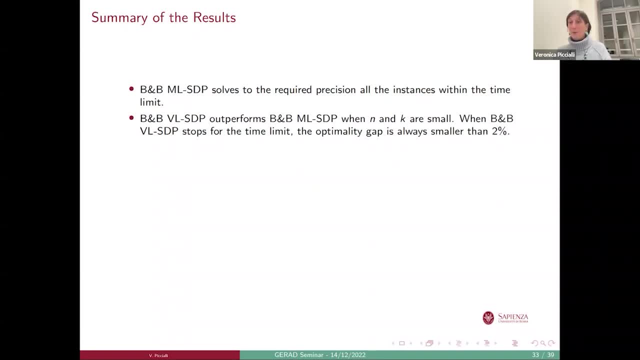 Because it outperforms in terms of time and number of nodes. the other one Because N and K are small And we know that the vector lifting relaxation- The vector lifting relaxation, is actually better. So we know that that's going to happen. 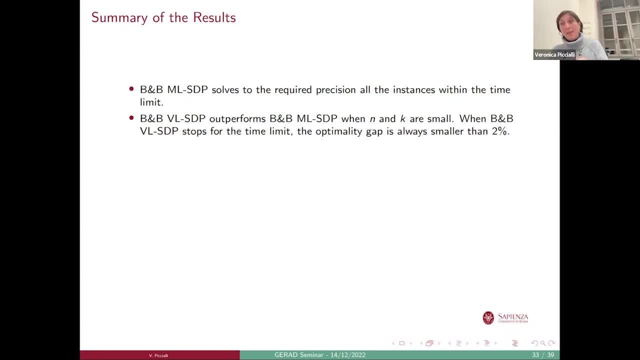 However, when the size grows, then in some cases the vector lifting as the branch and bound fails. But still the gap is always lower than 2%, So it still is not far away from the optimal solution. So what we can see is that the bound produced by the vector lifting relaxation is stronger and extremely tractable where N and K are small. 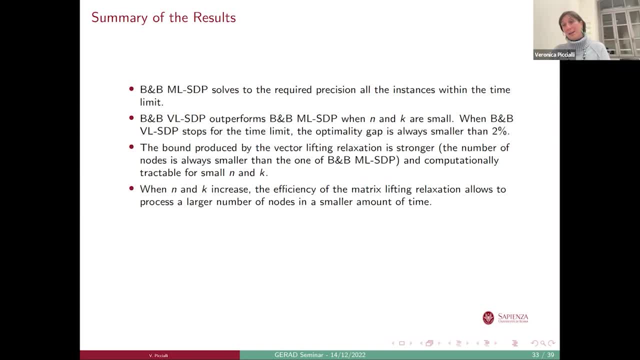 When N and K increase the efficiency of the matrix lifting. relaxation allows to process the larger number of nodes in a smaller amount of time, So it is able to close the gap And also keep in mind that we are using the size reduction And the size reduction is more effective on the matrix lifting version because we are doing more nodes. 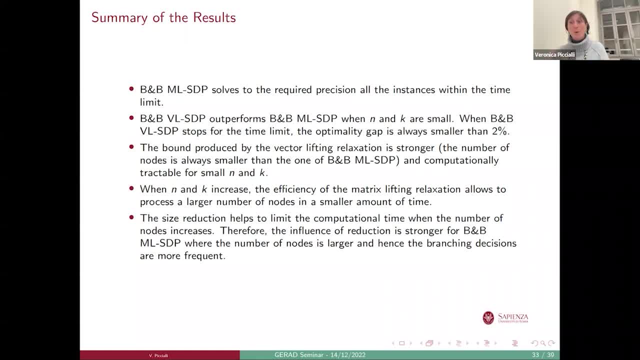 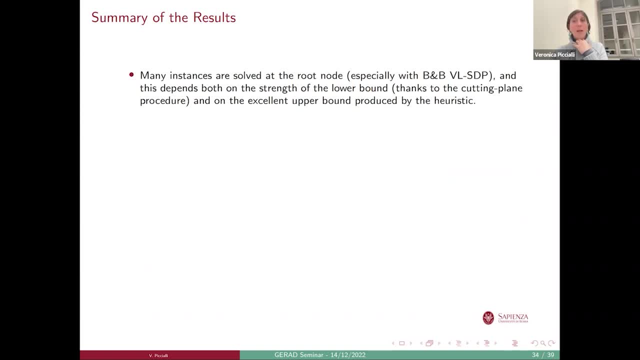 So we will have more branching decisions and we will have more masculine constraints, So the size of the SP field will reduce more. in this, in this case, So many instances have solved the root 2. Especially with the vector lifting, And this depends on the, on the one hand, on the strength of the lower bound and on the other, of how good the heuristic is. 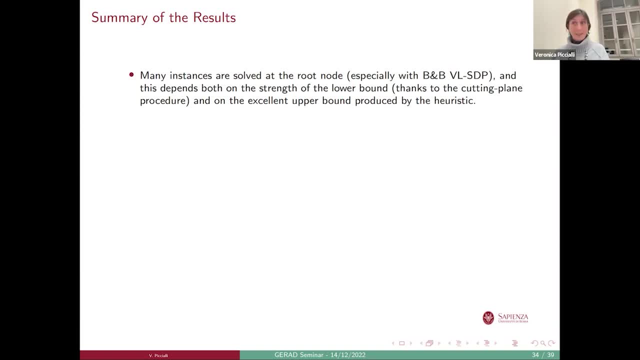 So it's not trivial here finding the global minimum in terms of the upper bound. also, And the statistics on the root node confirm us that the vector lifting relaxation is stronger. since it is tight, We actually do not need cutting plane iteration out of 29 instances. 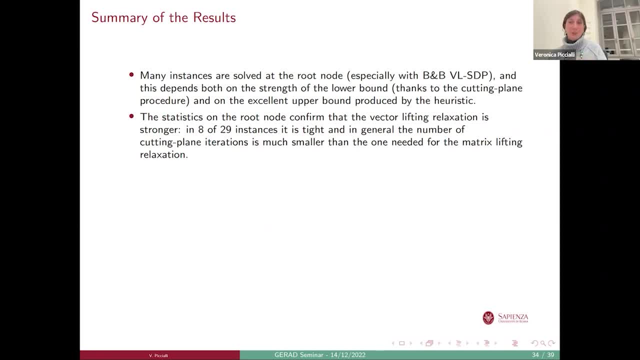 In general, the number of cutting plane iterations Is smaller. However, at the end of the root node, this difference that you can see in that get 0 after the captain plane iteration, this difference becomes almost negligible. So, and this is really thanks to the captain plane procedure, 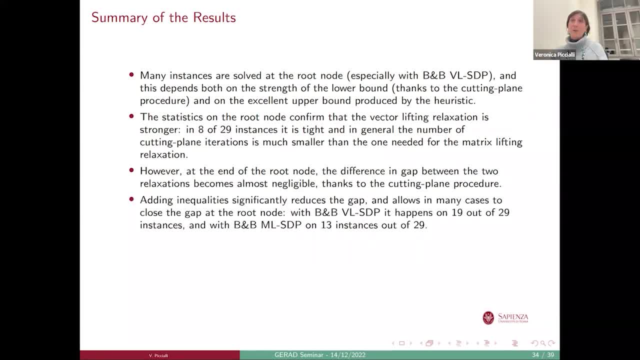 So adding inequalities really significantly reduces the gap. In many cases it allows us to solve the instances at the root node. When K increases, this relaxation in general become weaker. So when K, when K is larger than 4, actually it can happen that we can do not find the upper bounded root node. 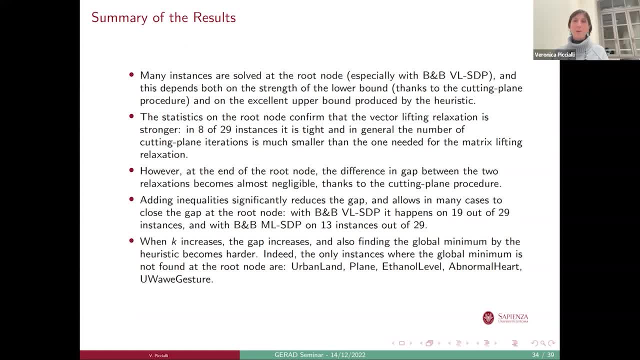 So it's not a matter of certifying the upper bound, but we really need to go down in the tree on the instances where K is larger in order to find the upper bound. So the the problems where K is larger becomes, the more difficult ones. 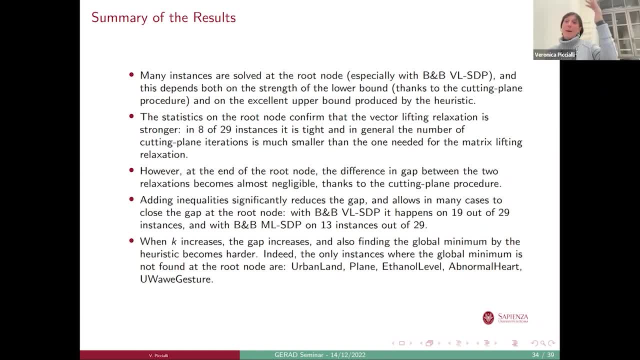 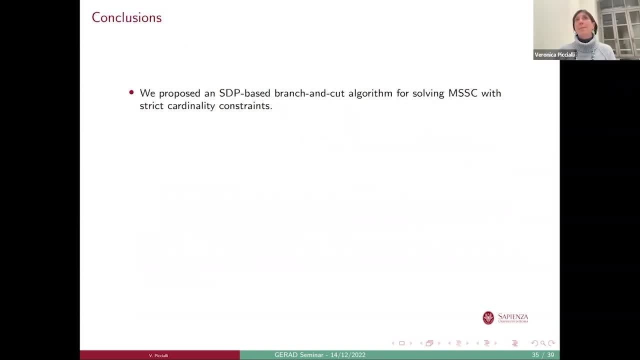 And in that cases you can see that you update the upper bound Many times when you go down the branch and boundary. So, in conclusion, we have proposed an SDP based branch and cut algorithm for the minimum sum of squared clustering with strict cardinality constraints. 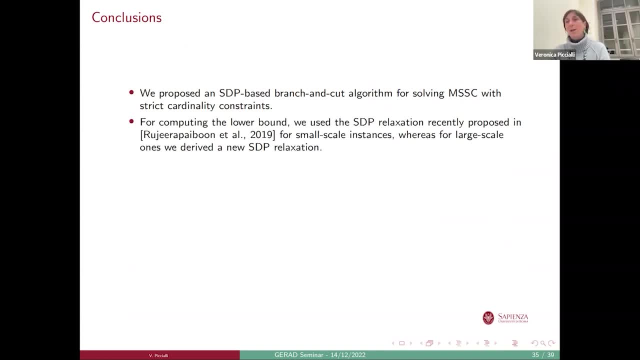 And we use the two different SDP: relaxation One works very well, which was known for small scale instances, whereas the one that we propose is slightly weaker. But is it more effective when the size increases? And implementing the cutting plane was fundamental for improving the bounds. 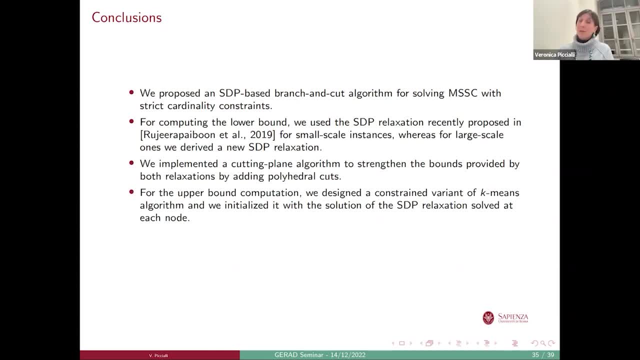 And also our heuristic, which is still based on the SDP, is extremely effective in computing a feasible clustering, constrained clustering and the numerical results. I didn't put the results against the competitor because the state of the art solver was only able to solve instances up to 200 points. 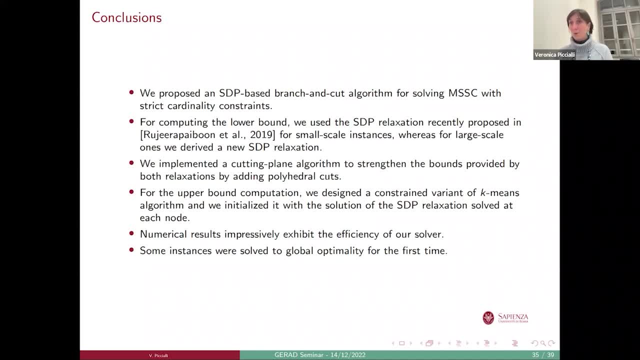 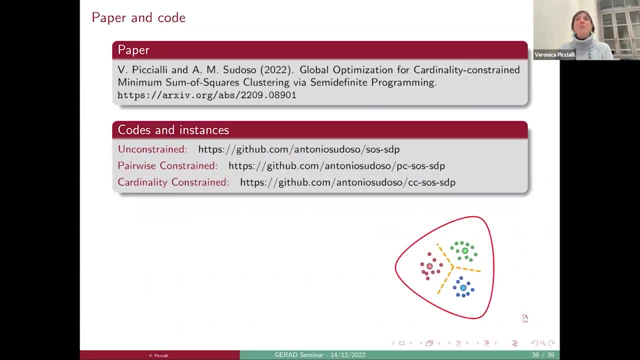 Most of these instances were never solved to global optimality before, So I didn't feel fair to put the table where we just win on all the instances, And so here you are. This is the paper There is an archive of about the cardinality version. 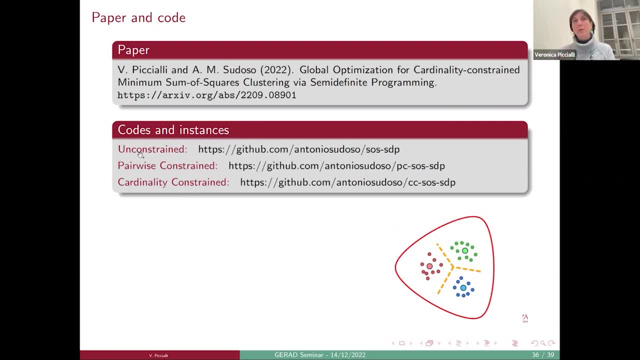 And these are the three codes that are all available on the page of Antonio, on the GitHub page of Antonio, for solving the three versions of the minimum sum of squared clustering, And then, after I have some references if you want future work, I didn't put the slide. 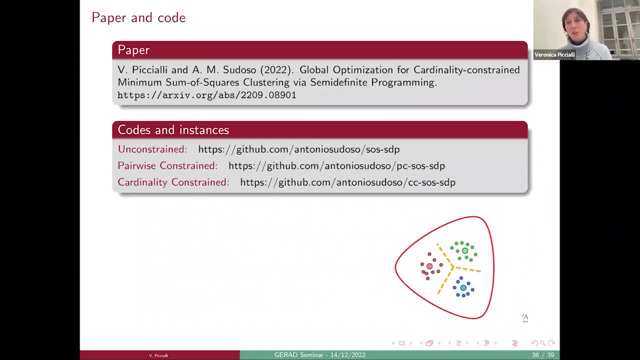 But the future work is to try to use this kind of exact approach for solving larger instances by doing some smart decomposition And in the smart decomposition trying to exploit the mastering constraints to reduce the size and see whether we managed to solve even larger instances.